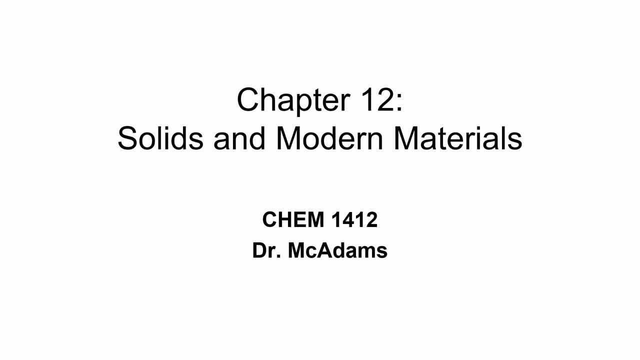 All right, so here's chapter 12.. We're only doing a few sections of chapter 12.. If you look at the learning objectives for chapter 12, you'll see that there's not very many, And so I try to address those learning objectives fairly briefly. There's a couple other things I like to point out, that's: 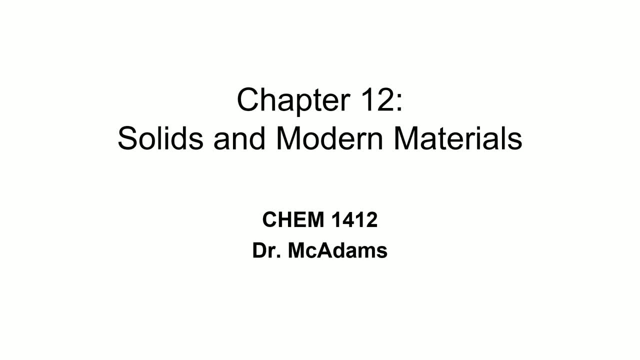 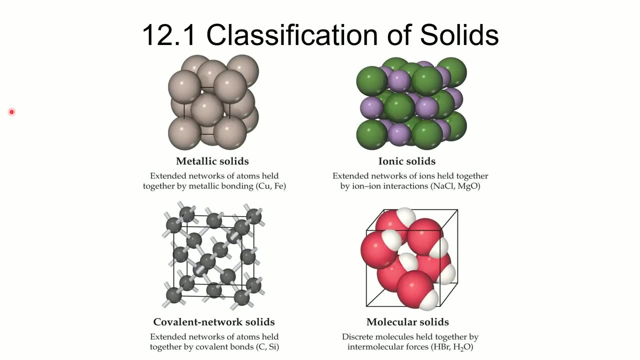 from chapter 12.. So we're not going to cover everything in chapter 12.. So just kind of keep that in mind. We're just going to be looking at a small segment. That's why I usually just kind of tag it on to the end of chapter 11.. So when we're classifying solids- one of the things that we like- 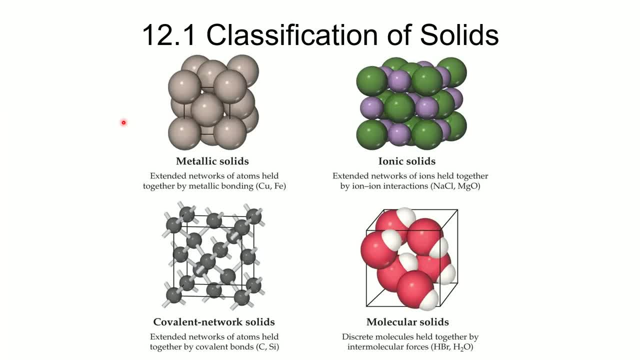 to do is to look at the different types of solids. What is it that's holding the particles together? We have metallic solids. These are pretty much any metal that you can think of- steel or silver, Gold or whatever- is going to have metallic bonds that hold it together. We'll talk about those in a 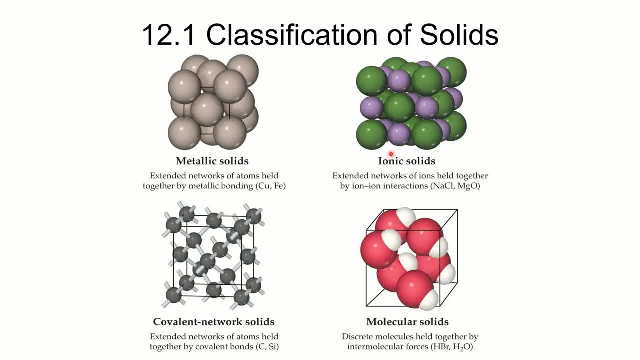 little bit more detail here in a bit. We have ionic solids. Those are held together by ionic bonds. Sodium chloride is a good example of that. We have covalent network solids. This is where the thing that's holding it together is going to be. the thing that's holding it together is going 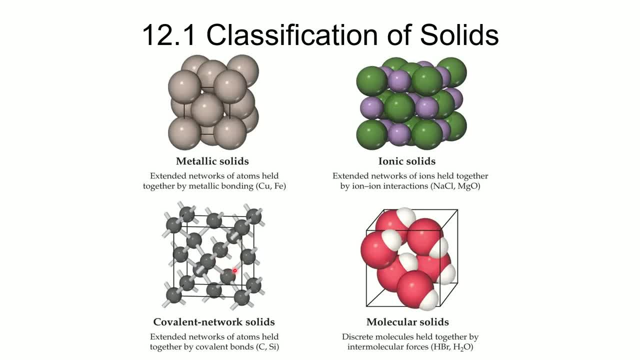 to be covalent bonds, And so diamond is an example of that, And I will show that to you here in just a moment. And then, finally, molecular solids, the thing that holds that together. those together are going to be intermolecular forces. 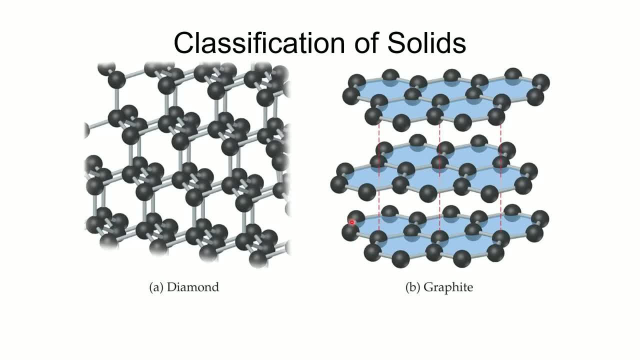 So here is an example of something to differentiate between a covalent network like diamond, which is very hard and very rigid, And then over here we've got a molecular solid Graphyte, which is also pure carbon, And it is much, much different. Now I don't have a diamond to. 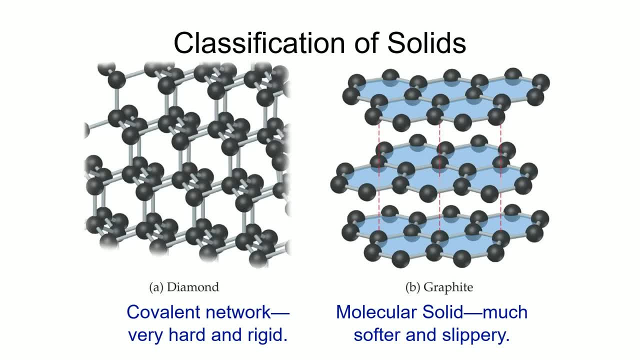 show you, but I do have some graphite to show you, So I'm just looking at a couple of differences here. If you look at the molecular structure, each of the carbons in that diamond is bonded to four other carbons, So each carbon is sp three hybridized. If you go back and look at chapter nine, you'll see that. 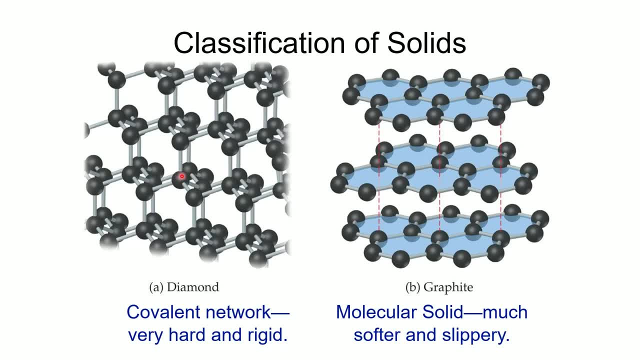 different carbon is bonded to four other carbons, So each carbon is sp three hybridized. If you go back and look at chapter, look at chapter nine, you can look at what SP three means again And uh, and so every one of 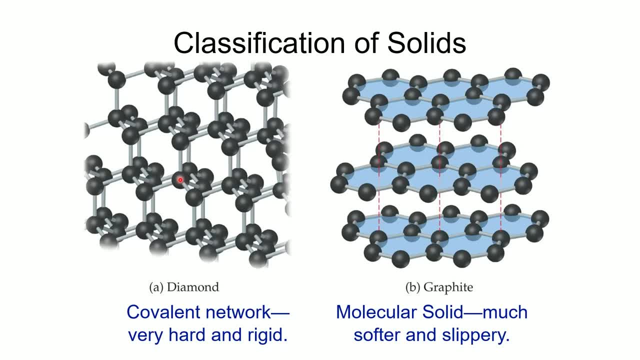 those carbons is locked into place by the bonds with the four carbons around it. As a consequence, we will find that that carbon, uh, that that structure for diamond is very rigid and very, very hard. Uh, diamond is one of the hardest substances known to humans, And um, in addition, 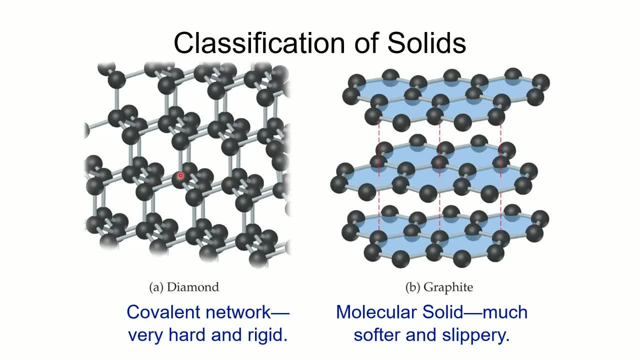 to being beautiful. uh, diamonds are also quite useful, uh, as an abrasive, because it's such a hard substance. Now, graphite, on the other hand- you'll see here, it says that it's uh much softer and slippery. Um, it has a very dark color to it. Uh, you'll notice that each of the carbons 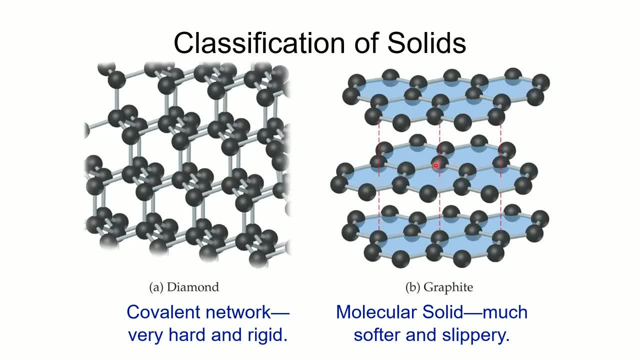 in graphite is SP two hybridized, So it's connected to three other carbons. Uh, but each of these sheets are can move past each other. So, uh, they, they can slide past each other relatively easily. So, um, I am going to. 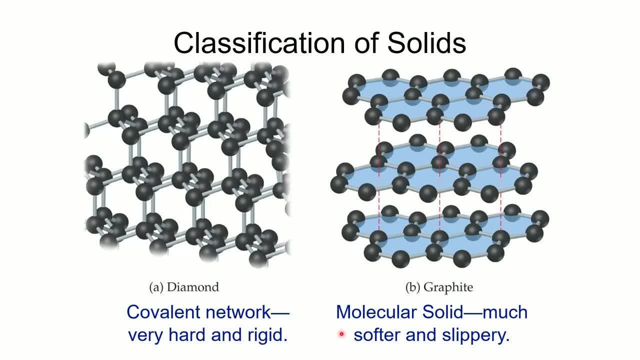 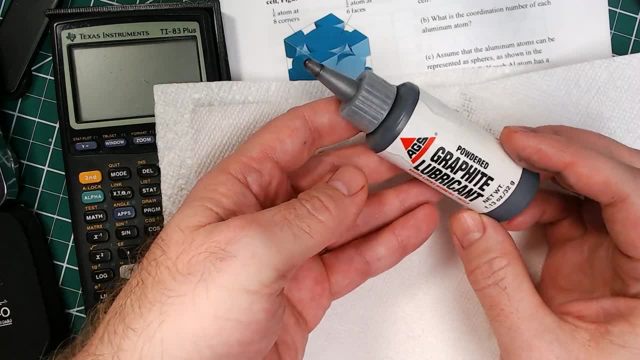 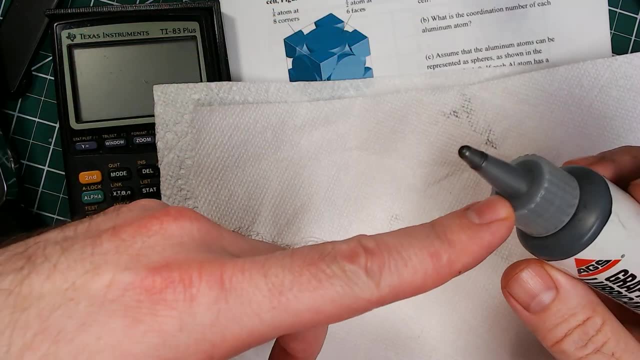 demonstrate this, what this looks like, by switching over. All right, So I've got a paper towel here, because this gets a little bit messy. So this is just graphite. It's used as a lubricant, If you put, if you uh squeeze a little, if you've got a lock, that's seized up if you squeeze a little. 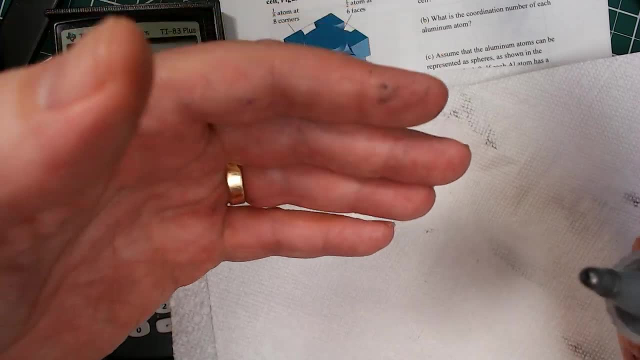 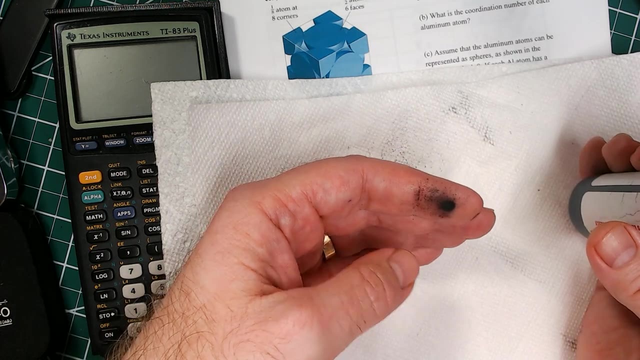 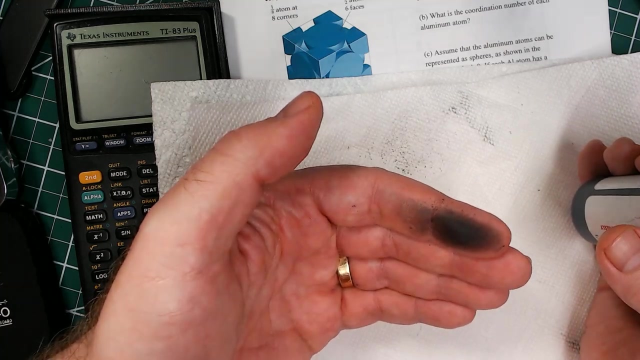 bit of this graphite powder into that lock. it helps to lubricate the lock. So I'm just going to there we go, That's plenty. So I put a little bit onto my finger and if you rub it you'll find that it is very soft and it's very slippery, And so, uh it, it actually makes kind of a mess. 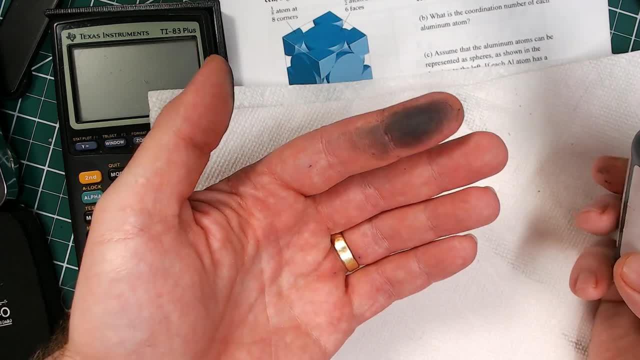 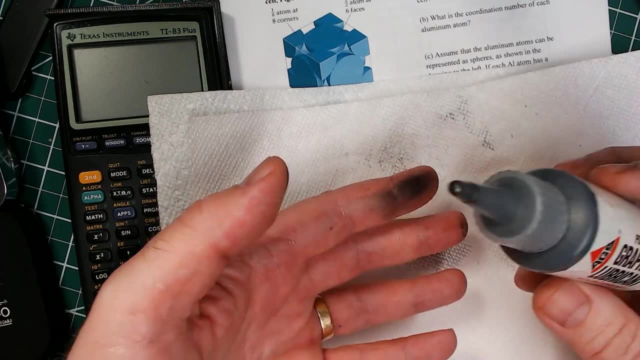 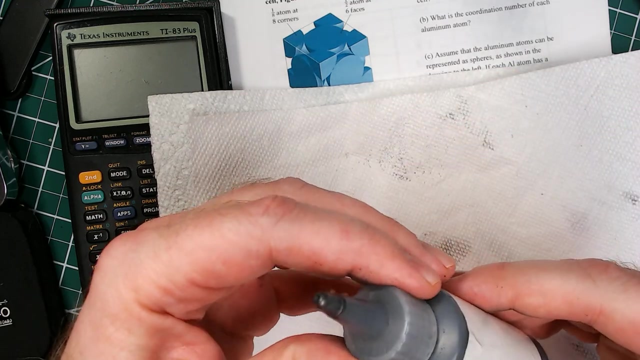 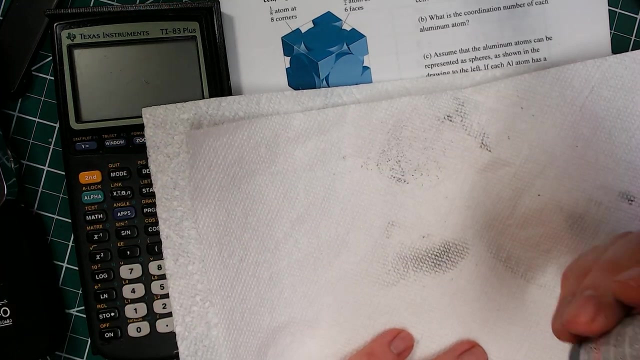 Um, graphite is the same substance that makes pencils work, So, uh, so that that's what the graphite's made out of. Um, but it turns out graphite is an excellent, excellent lubricant, because those sheets of carbon um are capable of sliding past each other. And, um, and also if you take, if you take something. 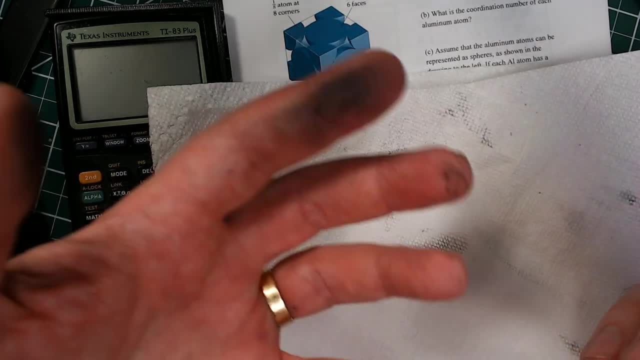 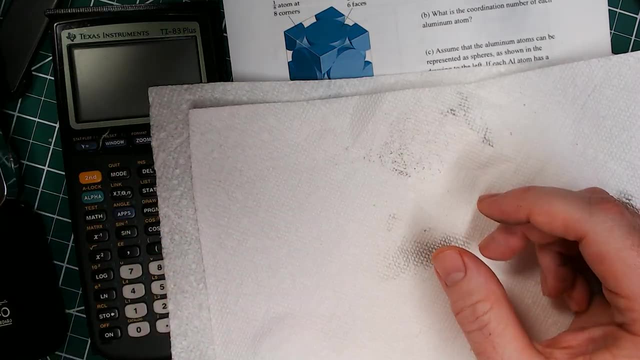 like oil or grease and put that into a lock, that can cause the lock to get all gunked up and uh, and graphite ends up being a much better choice for that. So graphite is pretty handy to have around. I've I've got some in my workshop all the time. I don't use it all the time. 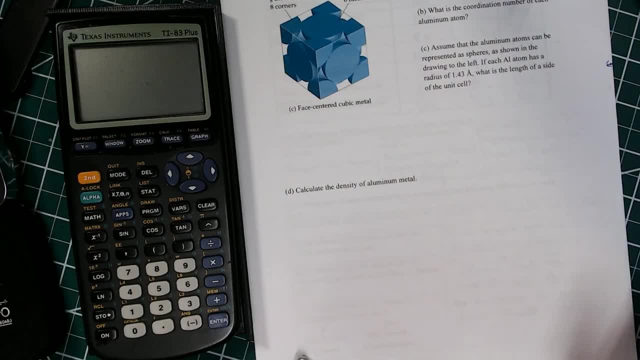 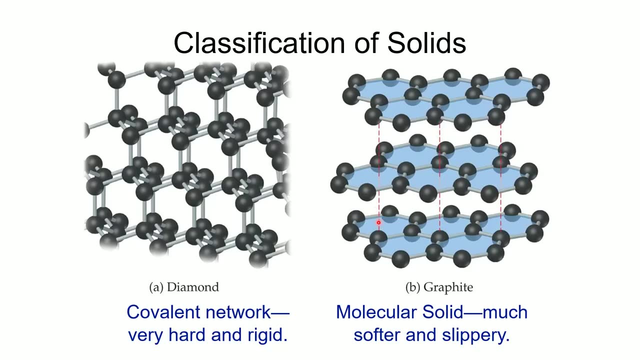 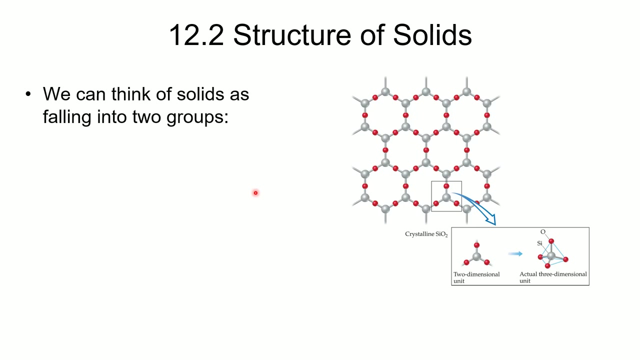 but I always have some ready to go, All right. So that's diamond versus graphite. When we're looking at solids, we can- we can categorize uh solids into being either crystalline, which is where they have a highly ordered arrangement over here on the right. Uh, we've got uh crystalline silicon dioxide, Um. 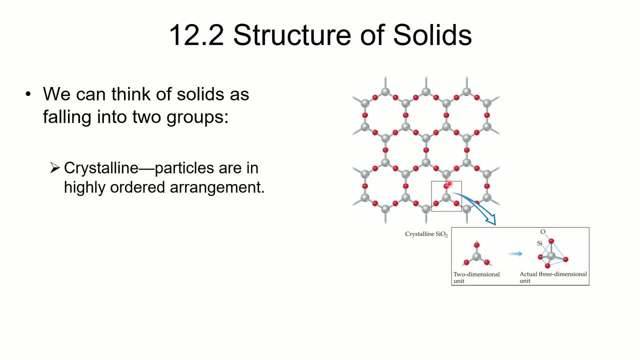 this is what we would see if we observed quartz: Uh, it's going to have a very regular structure. Uh, um, so it's going to have a very regular structure. Uh, um, so it's going to have a very regular structure. Uh, um, so you'll see that these atoms are, uh, these, what? 12 membered. 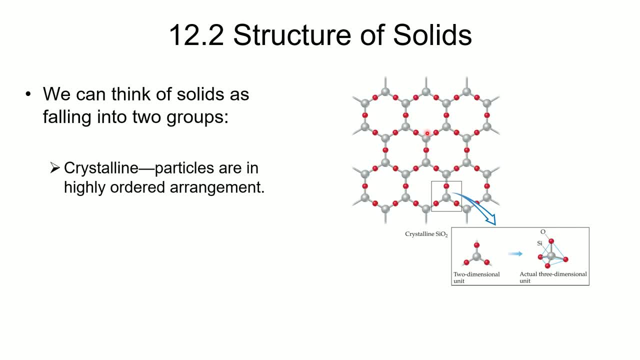 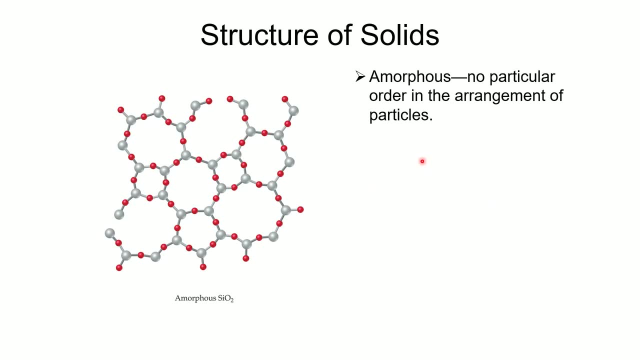 rings here. Uh, they're very regular and repeating And, as a consequence, they these form very nice, pretty crystals, Whereas if we take silicon dioxide and we heat it up in a different way, we'll find that we get- uh, we get- irregular, uh, uh, arrangements of the atoms. So we call 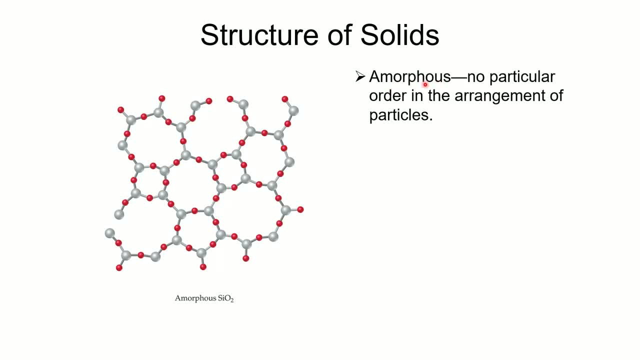 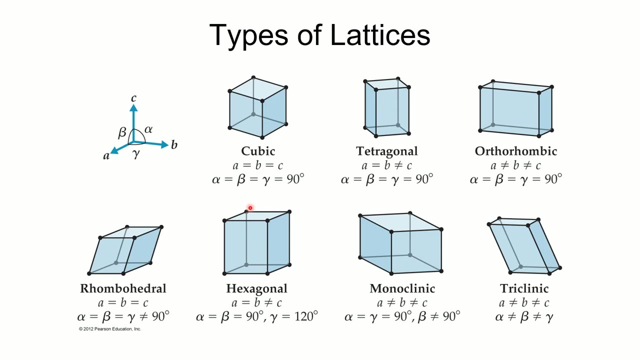 those amorphous, and amorphous just means without form, So amorphous solids, not crystalline. Uh, if you have silicon dioxide and it's amorphous, then that is going to be what glass is like. All right, So we're mostly interested in these crystals, and there are. 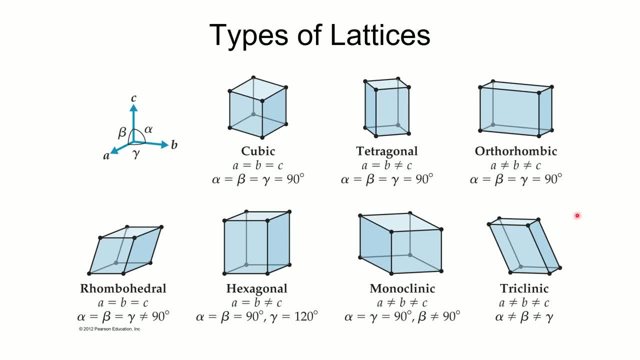 a lot of different possibilities for crystals, depending on the edge length, uh, for each of the sides, and the angles, And uh, and you'll notice that, as we go from one type to another, all that is changing is either one of the edge lengths is different. 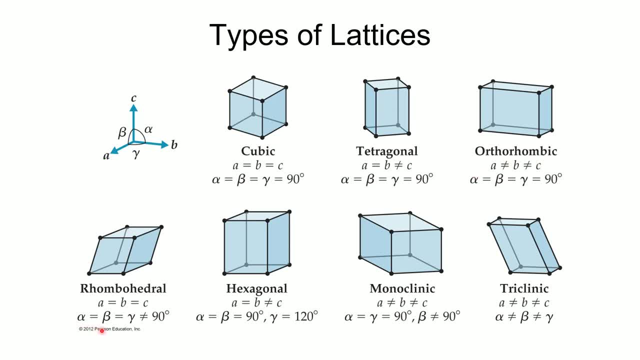 So like tetragonal versus orthorhombic, And if we come down here some of the angles, uh, the angles come out to different angles And so, uh, and then triclinic is going to be the one where 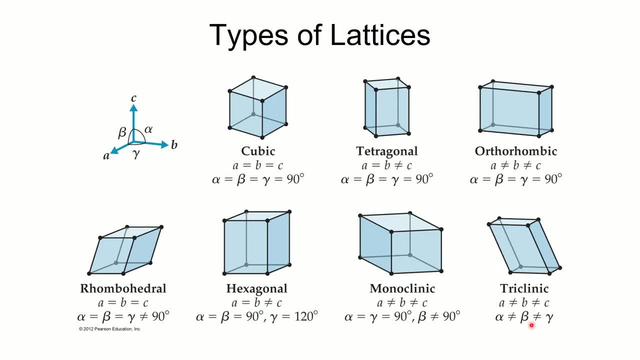 none of the none of the edge lengths are the same and none of the angles are the same, And so that's the most complicated In this textbook. we're going to be primarily concerned with cubic structures, And so we're simply going to look at cubic structures, All right. 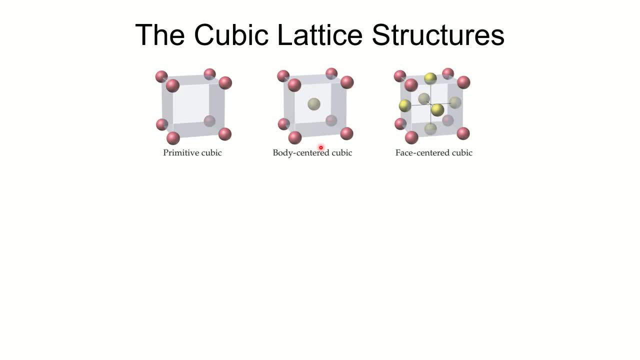 So when we're looking at the cubic lattice structures, there's three primary types that we're going to be interested in. We have primitive cubic, body centered cubic and face centered cubic. The primitive cubic will have one atom at each of the corners of that unit, cell Uh. 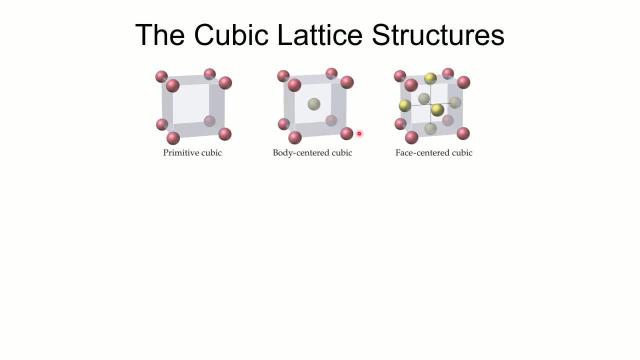 for body centered, we've got one of the atoms at each corner of the unit cell and then one in the middle. And for face centered, we've got uh one at each corner and we've got one one on each face. 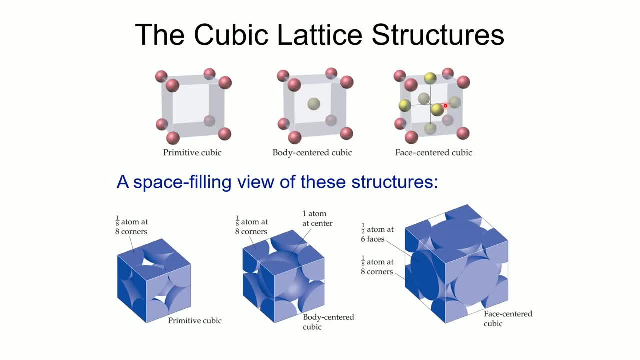 Now, if we use a space filling view of these models, so we have a space filling view of these models. this is what they would look like. We've cut off the other parts of the atoms that are in adjacent unit cells, and so you can see how much of each atom is in each cell. 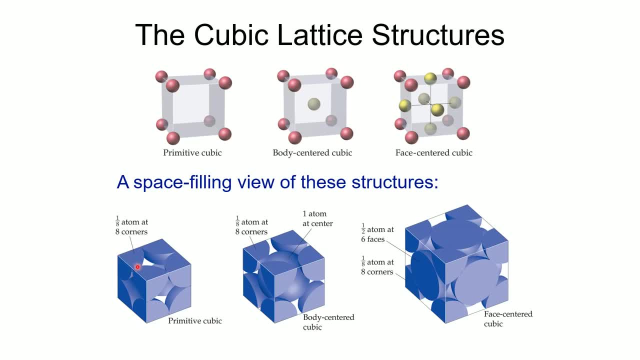 Dr Thomas Taylor, soon we'll notice that we have not creeped in very much. It seems like we need it a bit more often. Sell, You'll notice the atoms that are on the corner. One-eighth of the atom is within that cell And with that one-eighth of the atom within the cell and there's eight corners. Okay, Well, we Now we'll How many watands of the atoms in a cell. We would have about three quarters of an atom. Oh, one fourth. I was just calling each one. I'll do that One eighth. 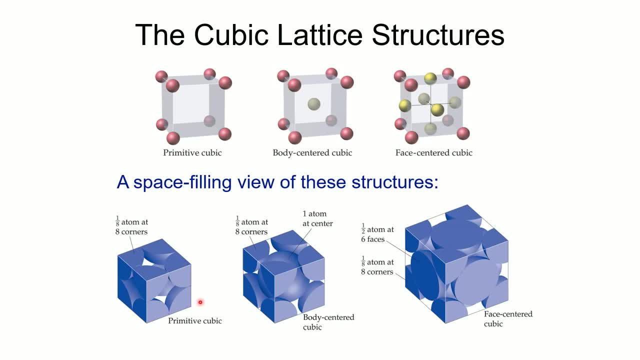 corners. that means there's one net atom in a primitive cubic crystals If we have a body centered cubic, so with body centered cubic we've got one atom that is in the middle And then we've got one eighth, that is at each of the eight corners, And so there's two atoms within that. 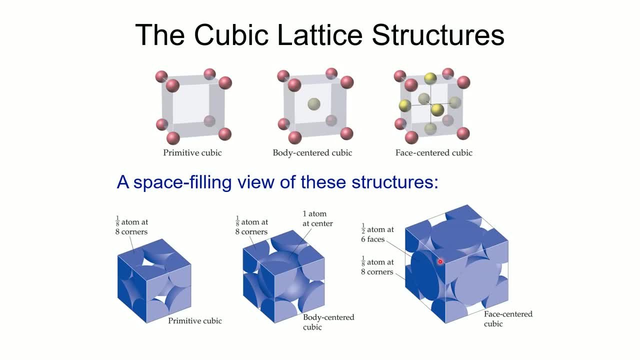 cell For face centered, you'll see that we've got one eighth of an atom that's at each of the corners And we've got half of an atom that is at each face. And so, since there are six faces, six times one half is three plus the one from the corners. that gives us four atoms that are: 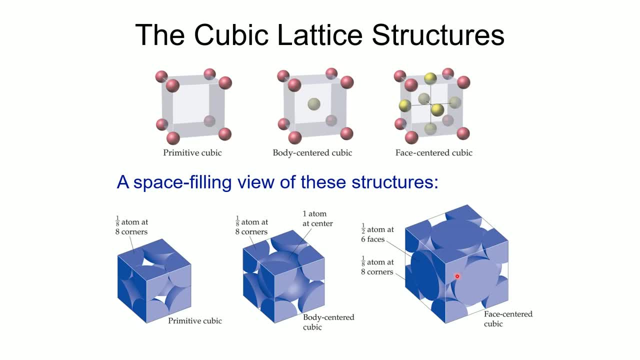 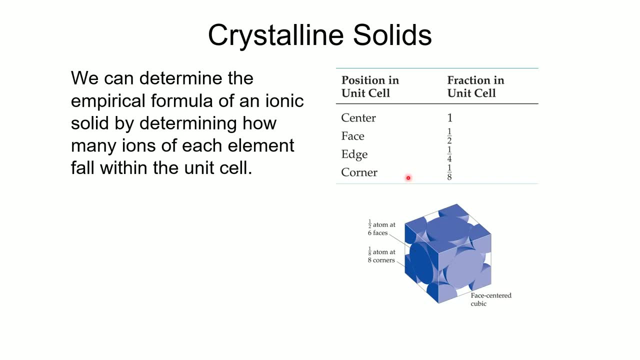 within a face centered cubic, All right Now. we've seen center, face and corner. We haven't seen any edge. We don't see edge with these three cubic structures. If we had a rectangular one instead of cubic, it is possible to have edge atoms And in that case 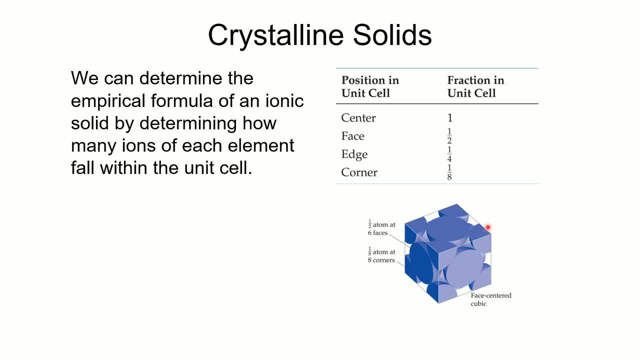 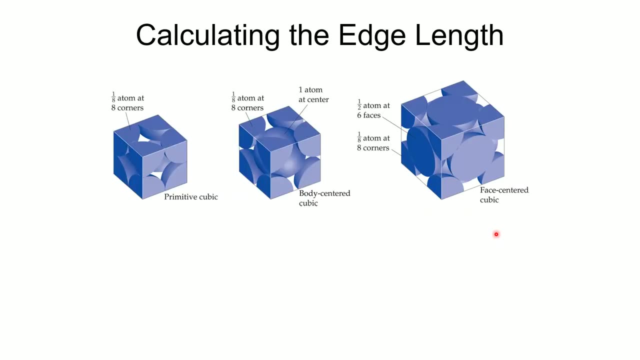 we'd have. one fourth of the atom is present. So with this information and knowing that these atoms are in contact with each other, there's a little bit of extra information that we can get about these unit cells, All right. So if we know the radius, we can get the edge length, And if we know the edge length, 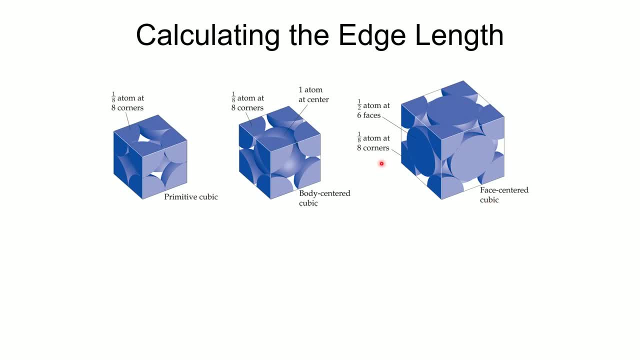 we can get the radius, provided that we know what type of cell is present. So if we want to look here, the edge length A, that is, the edge length A is from one corner down to another corner, And for primitive it's very easy, Since this is equal to one radius. 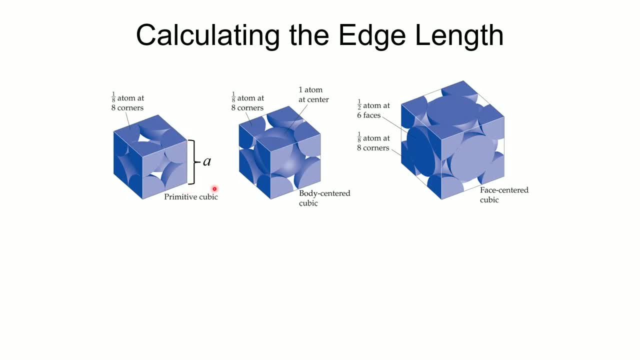 and this is equal to one radius, then that distance would be two radii, So it would be two R. So that equation is pretty easy. For a body centered, the math is a little bit more complicated. It's not too bad. You have to do the Pythagorean theorem twice in order to get this. But when you 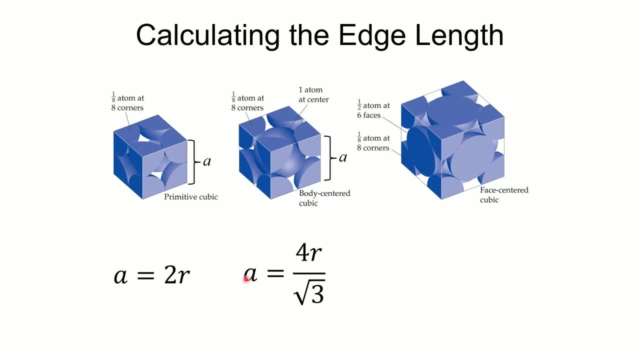 do that, you will get this: that the edge length A is equal to four R over the square root of three. And so that is for body centered And then for face centered. for face centered the math is a little bit easier. You only have: 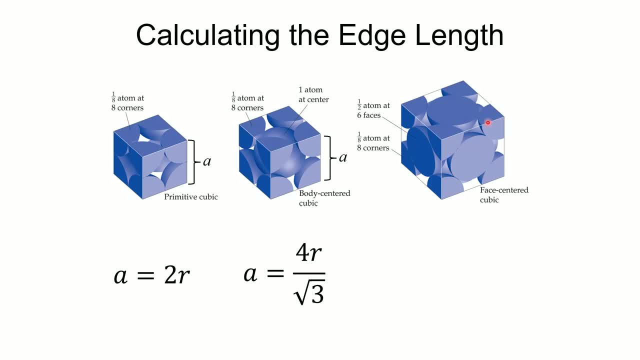 to do. you only have to do the Pythagorean theorem once. But the distance from this corner over to here is equal to four R. And since that's equal to four R and each of these is A, you plug that into the equation and you can solve for A and you can get. A is equal to four R. 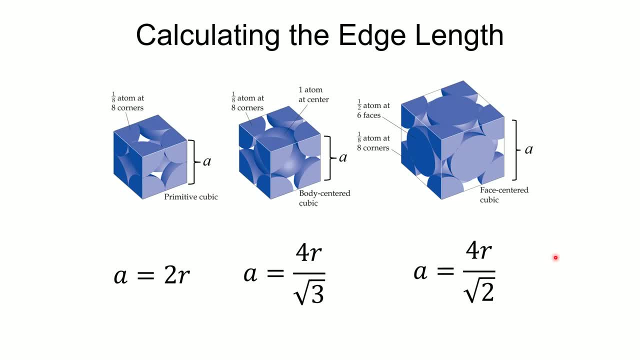 over the square root of two. We can use these numbers to calculate edge length, if we know the radius, and the radius if we know the edge length, And we can even calculate the density of a particular metal given this information. So we're going to go to number 62, and this is the last one. It's actually chapter 12 instead of 11,. 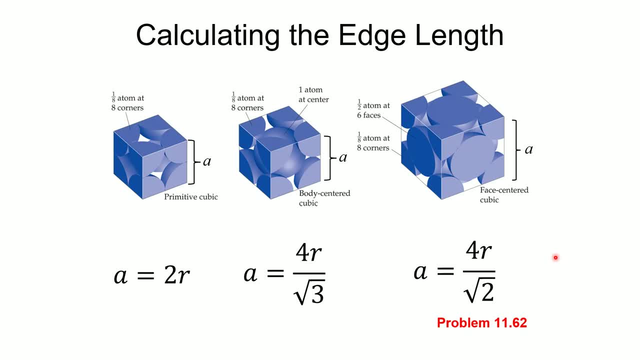 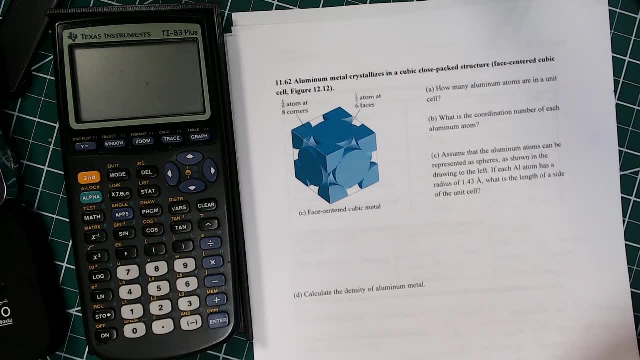 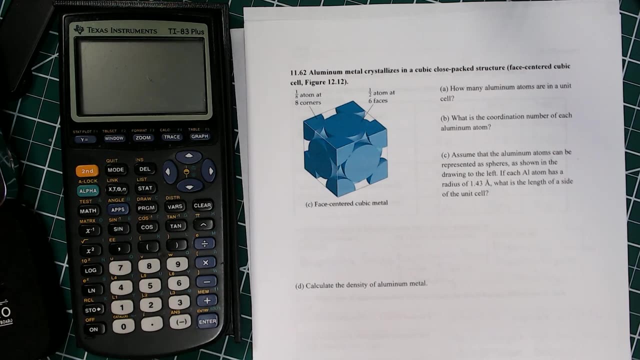 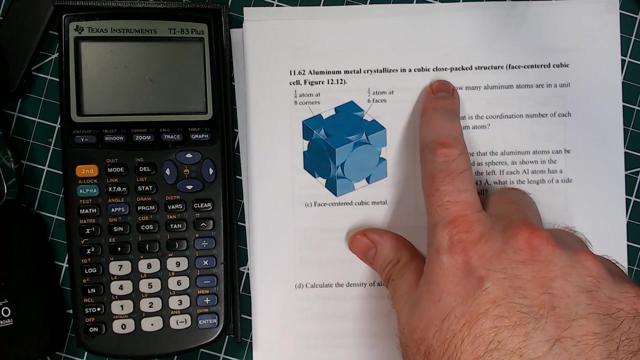 but oh well, All right, So I still have graphite all over my hands here, but that's okay. Make sure that that is all looking good there, Okay. So now what we want to do is we want to. we've got a face centered, So face centered cubic for aluminum metal. How many aluminum atoms are? 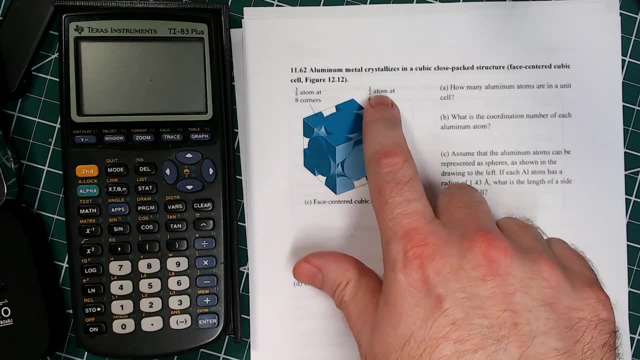 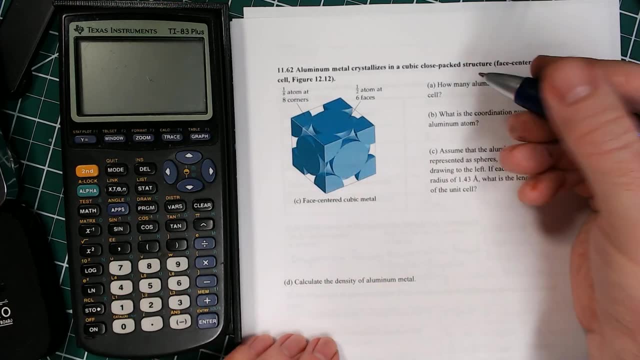 within a unit cell. Well again, if we've got six faces times four, we've got a face centered cubic. 1 half, that's equal to 3, and 1 eighth times 8, that is equal to 1.. So 6 times 1 half plus 8, 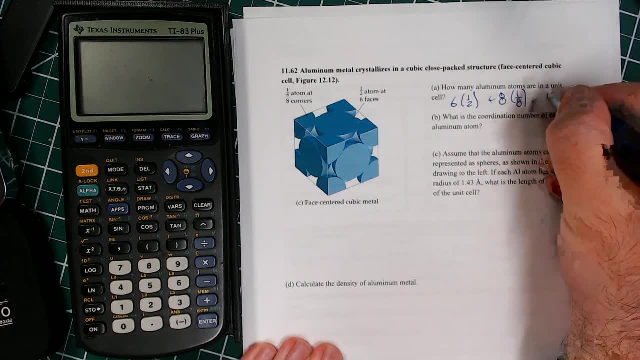 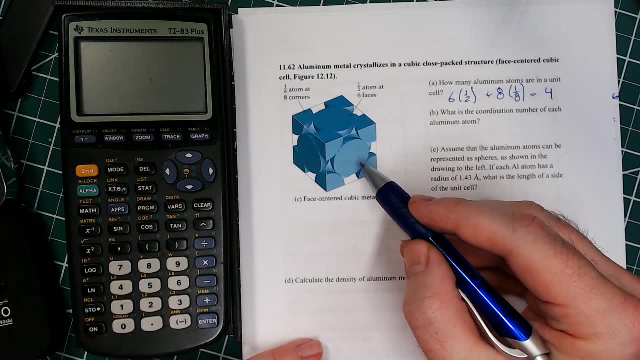 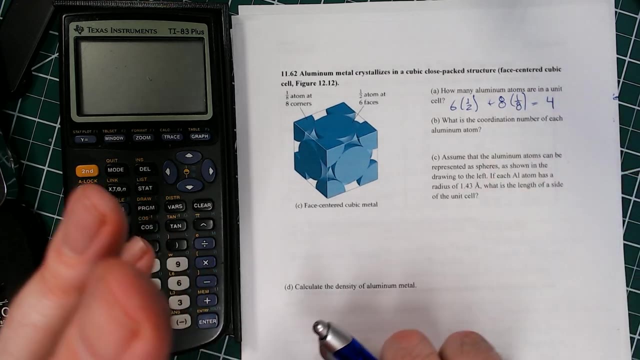 times 1, eighth, that comes out to 4.. So there are four net aluminum atoms within a unit cell of a face-centered cubic. All right, what is the coordination number? Now, coordination number: this is not a learning objective, so this is not something that you have to know how to do. 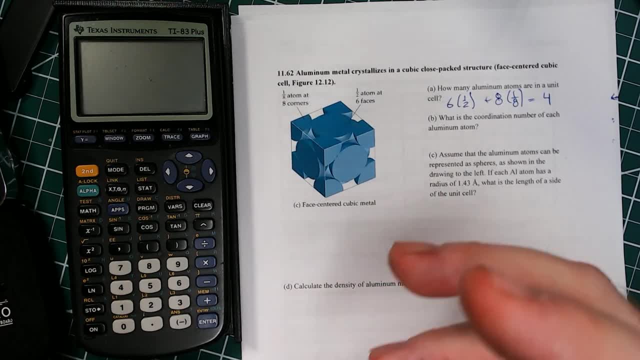 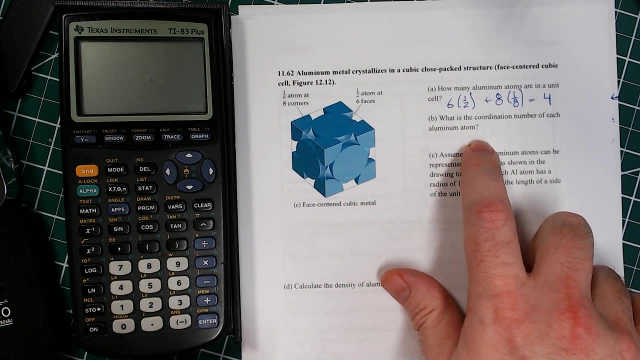 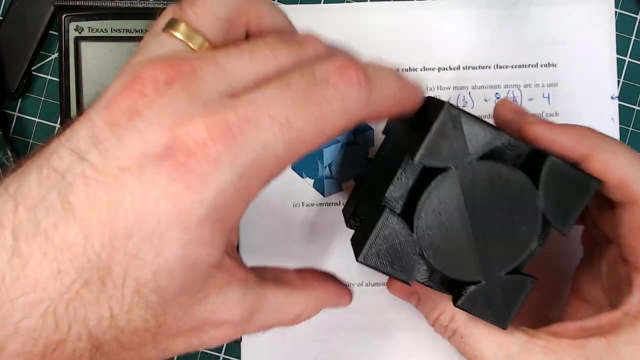 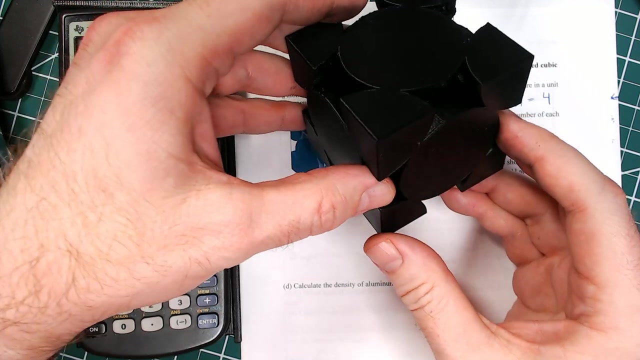 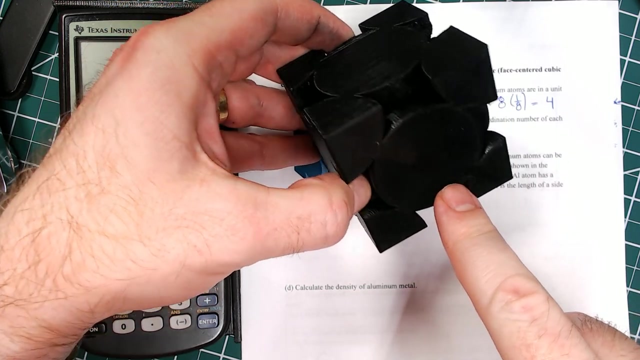 but it is interesting, So I'm going to go ahead and show you how to do the coordination number. All right, so I've got a 3D printed face-centered cubic. I 3D printed this one at my own house. so here's my 3D printed face-centered cubic. and we want to know how many atoms is one atom? 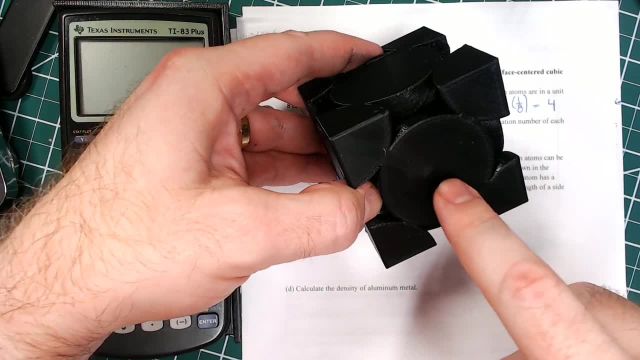 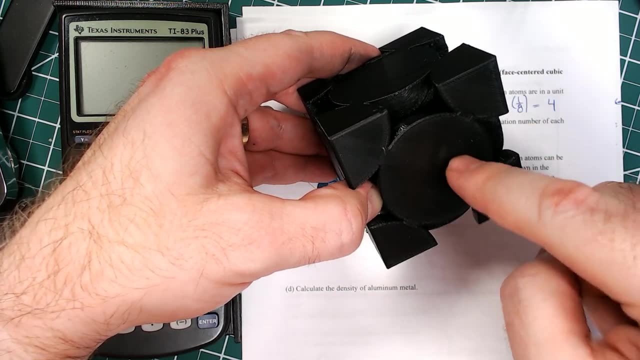 at the face here in contact with. Well, we can clearly see that this atom right here is in contact with these four. so that's 1,, 2,, 3, 4.. All right, this one is also in contact with. 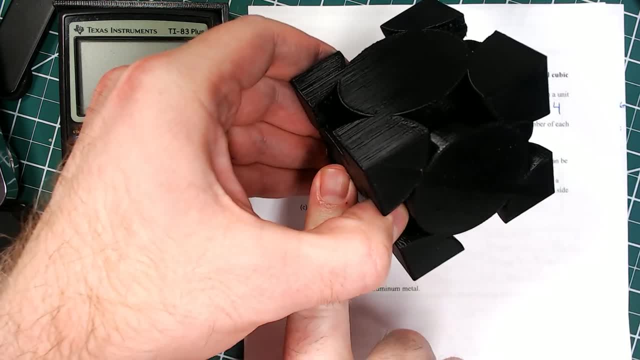 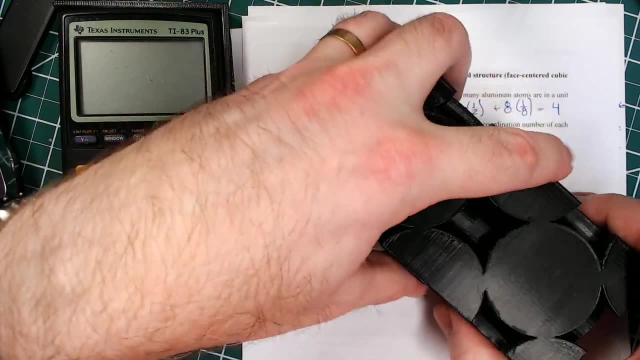 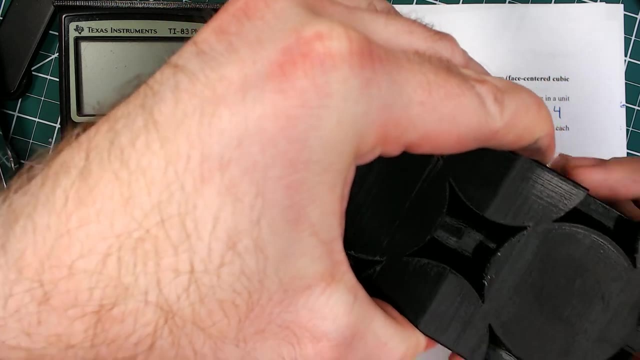 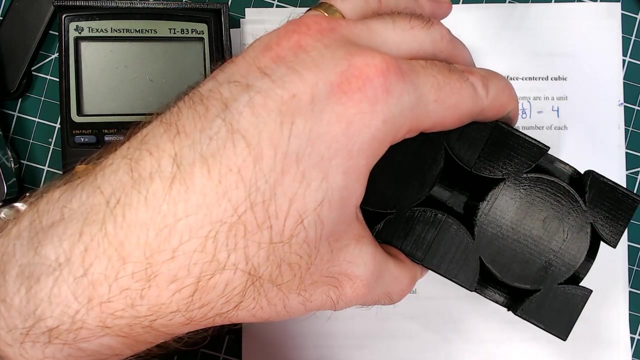 the adjacent faces. so 1,, 2,, 3,, 4 more, so that's 8.. All right, and so now this one is also in contact with the four that are on the adjacent faces over here. So that means 4 plus 4 plus 4, the coordination number is equal to 12.. So the 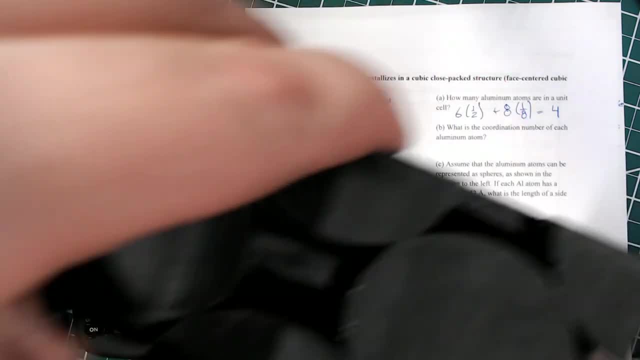 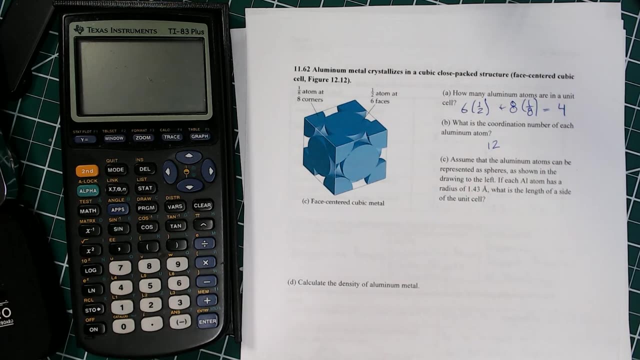 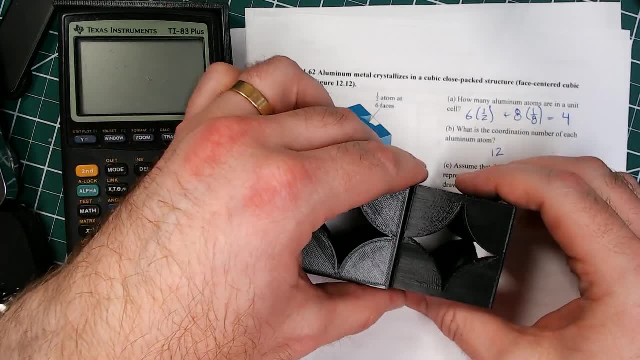 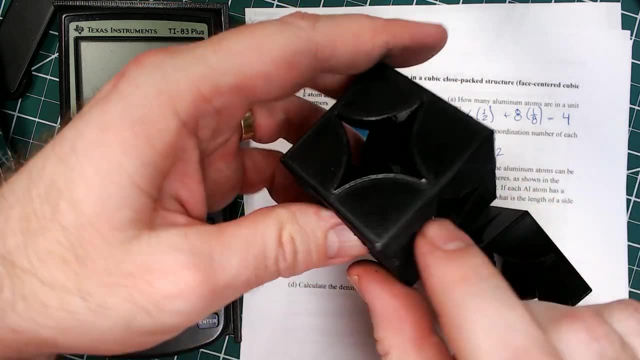 So here's the coordination number for some of these other ones, Like, for example, our point N, primitive cubic. well, for primitive cubic, this one's pretty straightforward, all right. so so here, if we look at this one, we can clearly see that this one, that's 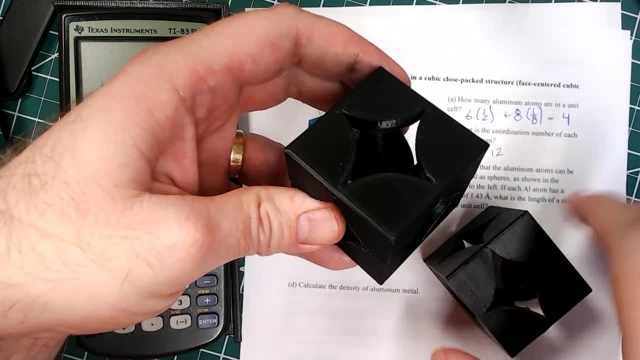 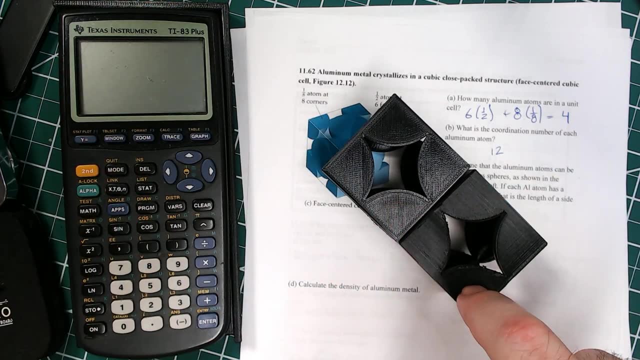 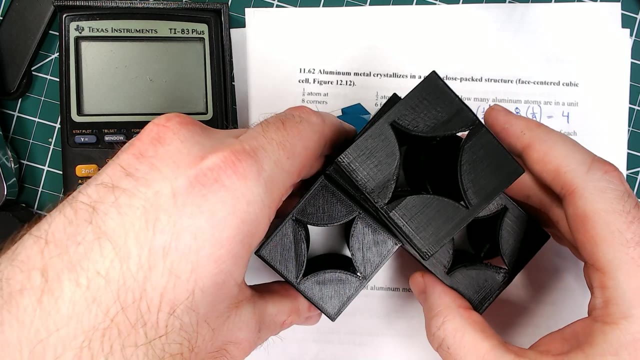 on the corner is in contact with one, two, three, but it is also in contact. so again, we're looking at this atom right here, it is in contact with this one over here and I've got a couple more here, all right. so again, a little bit difficult to. 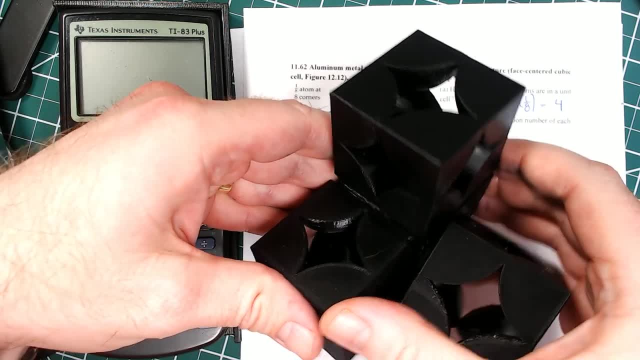 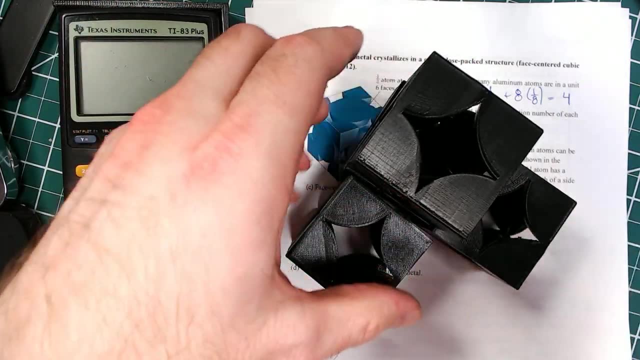 see because of the angle there. so it's in contact with one here, one there and one there, all right. so this- this would be a little bit easier to see if I wasn't trying to tilt it, but the point is that it isn't. it has a coordination. 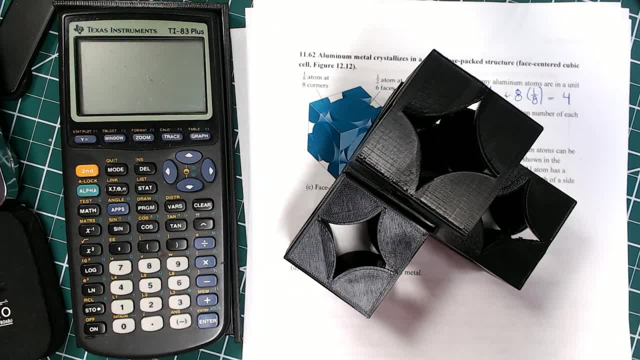 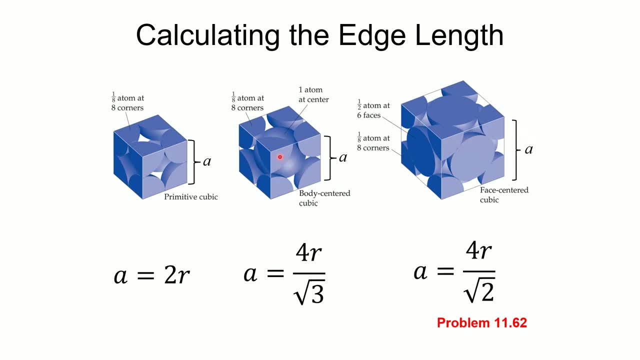 number of six. so if we go back and look over here- this one coordination number of six and this one a coordination number of 12, and this one a coordination number of 12 and this one a coordination number of 12, we think this one's got to be right in between, maybe nine, yeah, it's eight, but 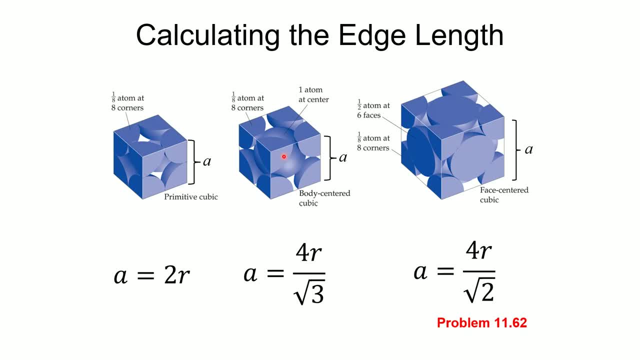 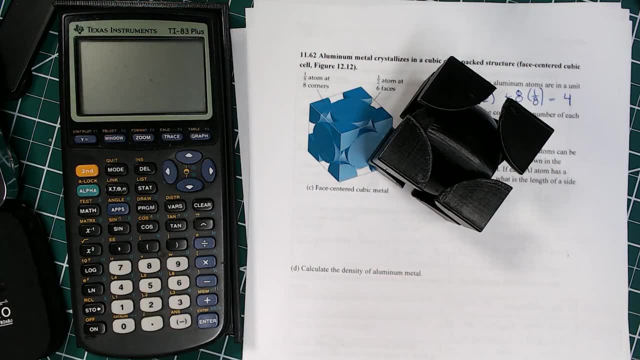 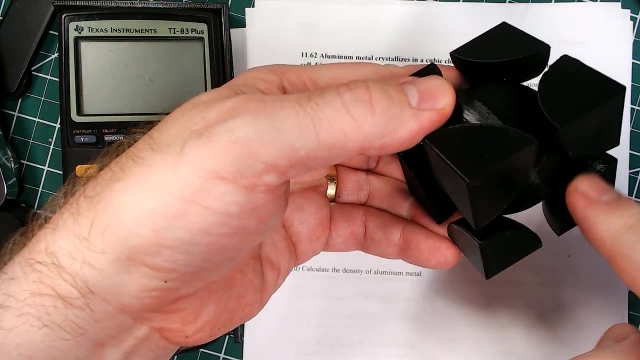 that one's actually easier to see, and and so I'm going to go back over here and I've got a body, centered cubic, here that I've printed out, and if you look at that body, uh, that one that's in the middle, it is in contact with all four of 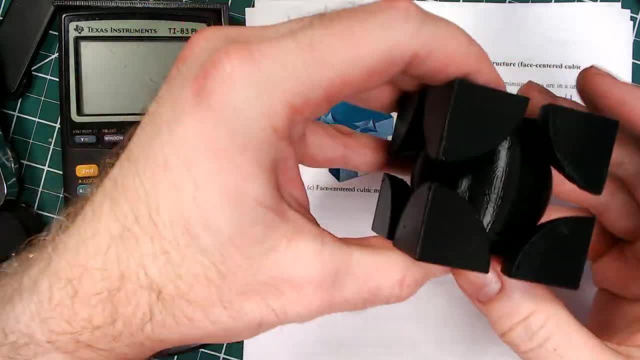 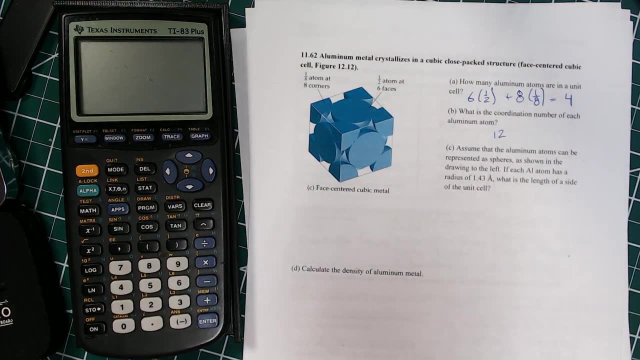 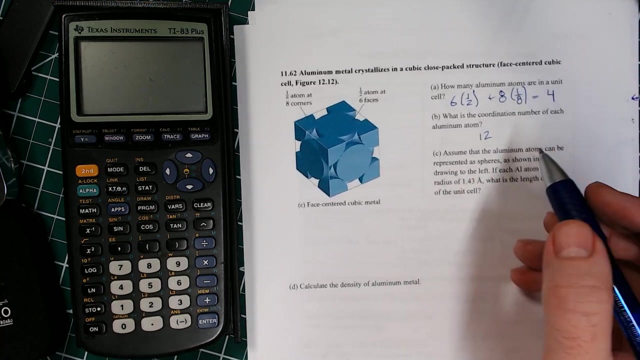 these and in contact with all four of those, and so that has a coordination number of eight again. I don't want to spend too much time talking about coordination numbers because coordination numbers are not a learning objective, but it is kind of interesting, all right. so assume the aluminum atoms can be represented as spheres as shown here, if each 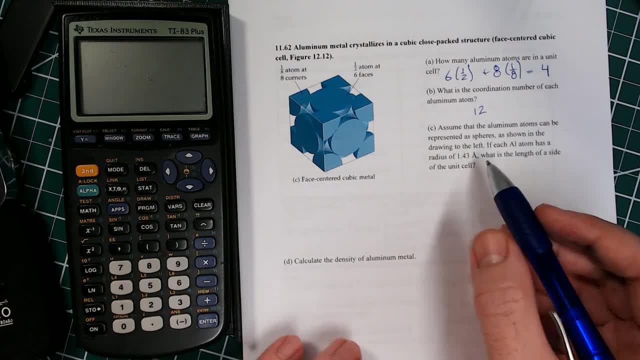 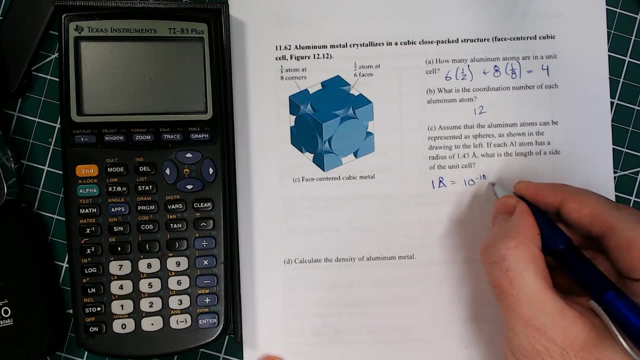 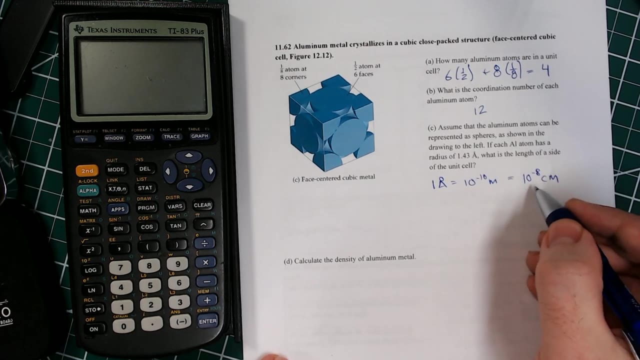 aluminum atom has a radius of 1.43 angstroms. just as a reminder, one angstrom is equal to 10 to the negative 10 meters, which is also equal to 10 to the negative 8 centimeters. now we're going to use that. 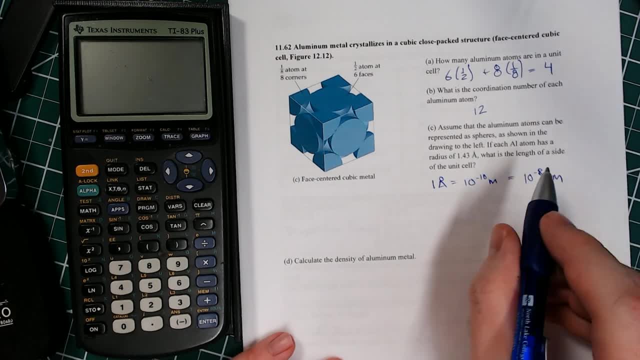 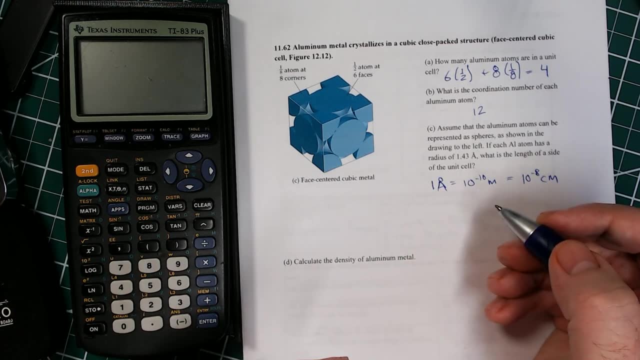 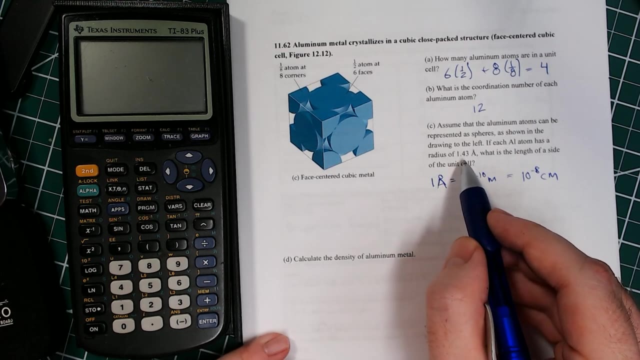 centimeter thing here in just a moment when we're doing our calculation of density, but that's just a reminder. turns out angstroms are a really useful unit for measuring Bond distances. so if each aluminum has a radius of 1.43 angstroms, what is the length of a side of the unit cell all? 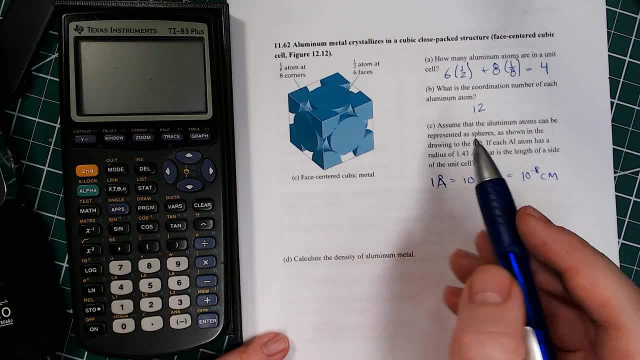 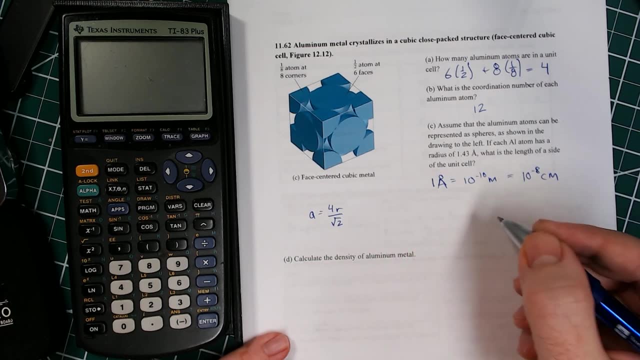 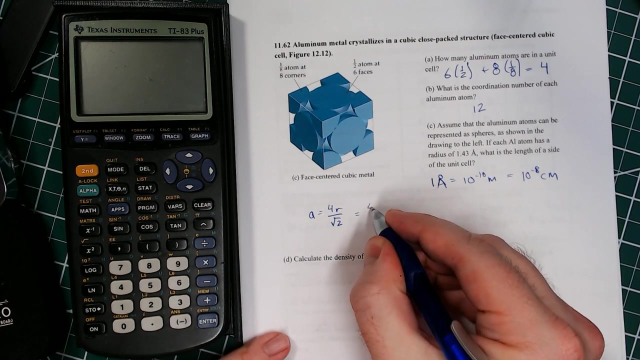 right. well, since this is face centered on this, a is equal to 4r over the square root of two. remember those three equations that I showed you. I recommend just memorizing those equations which one goes with which. all right. so a is equal to 4r over the square root of two, so four times 1.43. 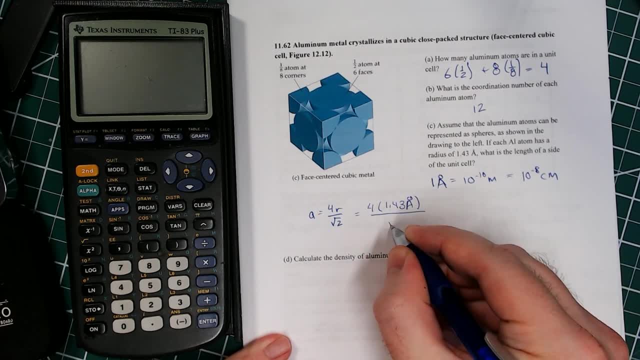 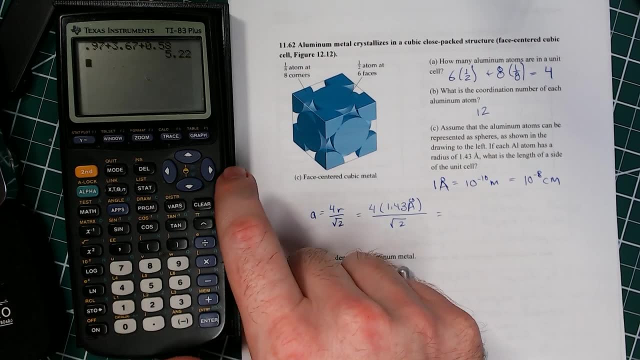 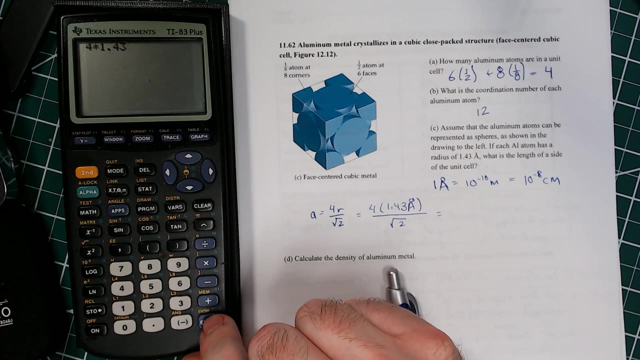 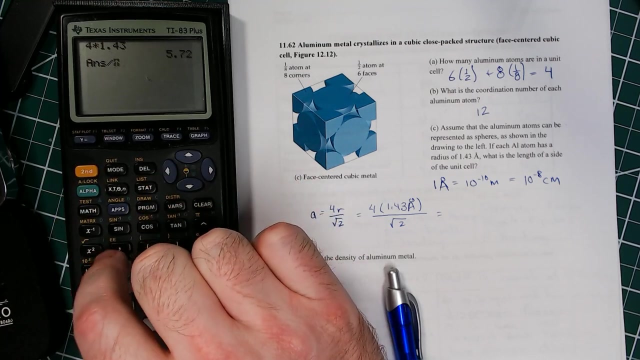 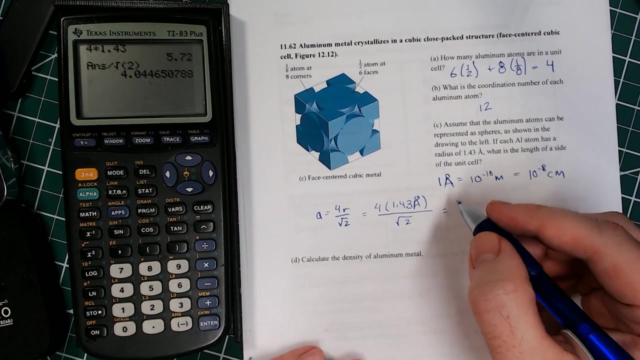 angstroms. divided by the square root of two, that comes out to a pretty easy calculation and we'll punch that into our calculator here. so four times 1.43, all right, and we'll divide by the square root of two and that gives us 4.044. since we have three sig figs, we're going to write that down is 4.04. 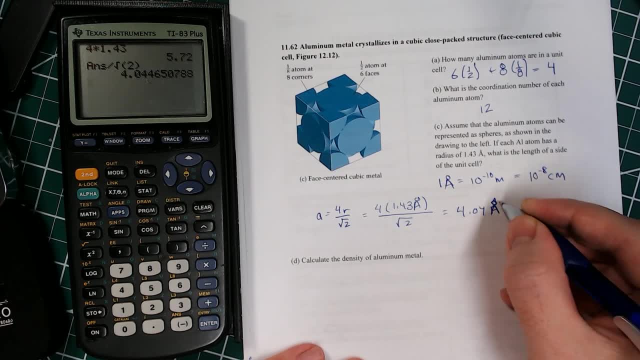 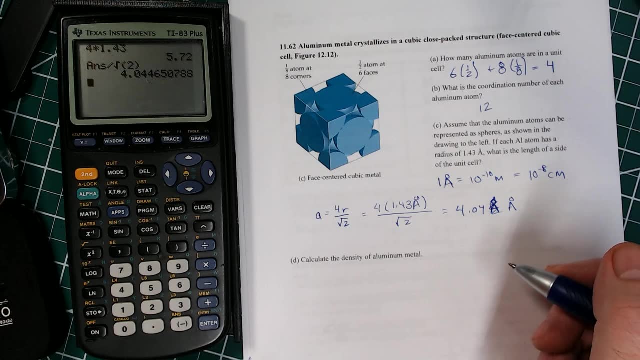 angstroms. so 4.04 angstroms there. my angstrom got a little weird there. let's try that again. close enough, close enough, all right, so 4.04 angstroms. so finally we want to calculate. so that means this edge length. 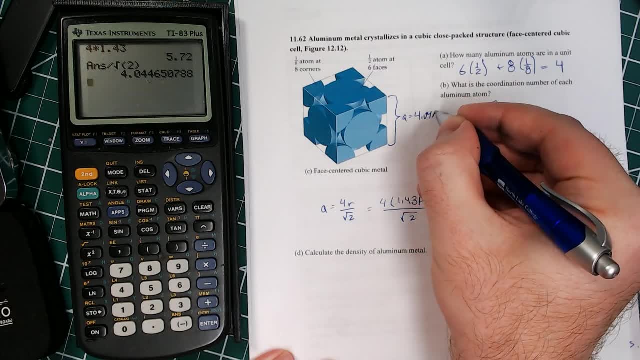 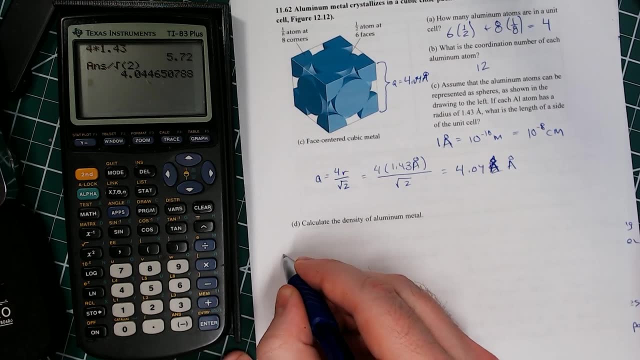 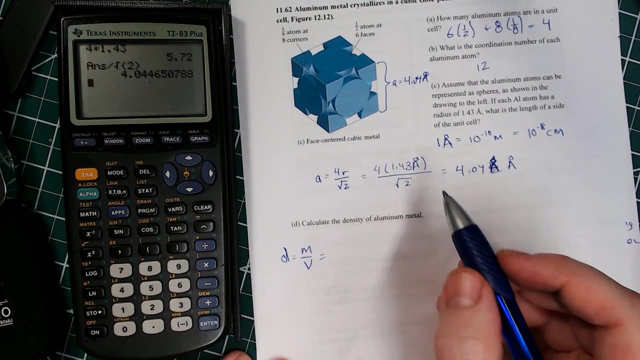 4.04 angstroms. all right, so now we want to calculate the density of aluminum metal. well, density is equal to the mass divided by the volume, the mass we're going to do the mass of one unit cell. so in one unit cell there are four aluminum atoms. 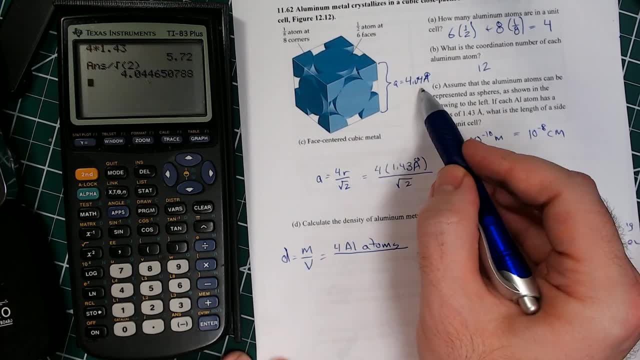 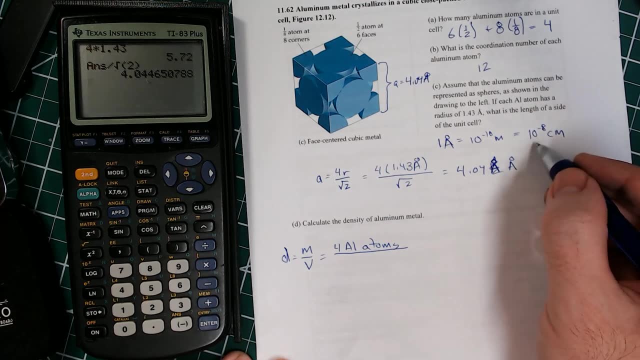 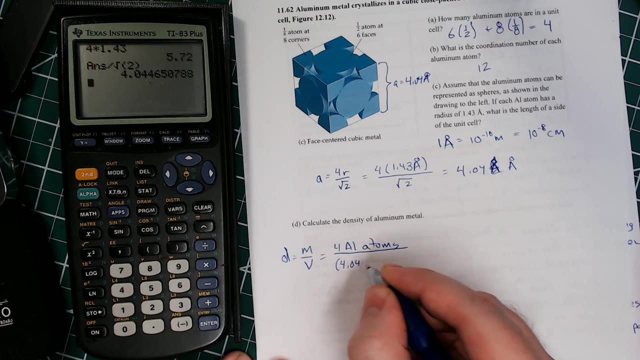 and then the volume. since this is cubic, we can just take this number and cube it, but instead of putting down 4.04 angstroms in place of angstroms, I'm going to put times 10 to the negative 8 centimeters. so I'm going to put 4.04 times 10 to the negative 8 centimeters. 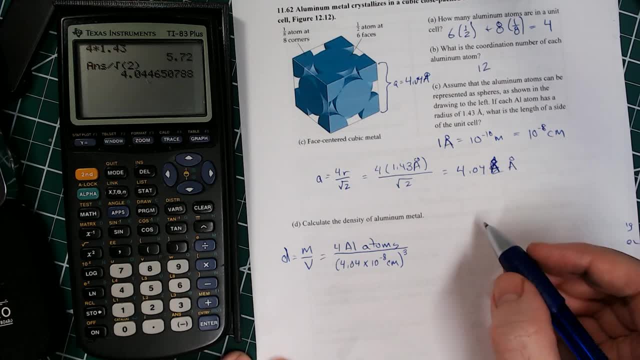 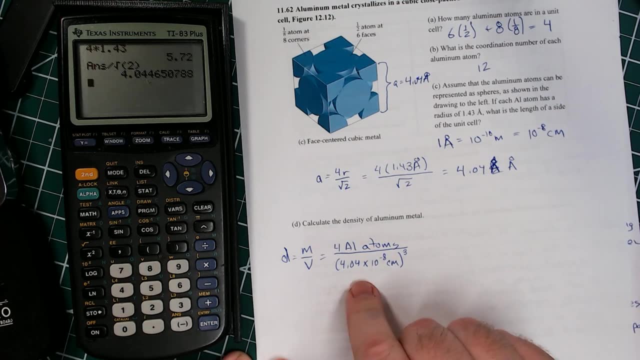 and then we'll do cubed. all right, so that's going to give us centimeters cubed down in the denominator. now, that's going to be a ridiculously small number when we cube that, but we've only got four atoms, so it'll all work out. To get from atoms to moles and then moles to mass. well, first we want to 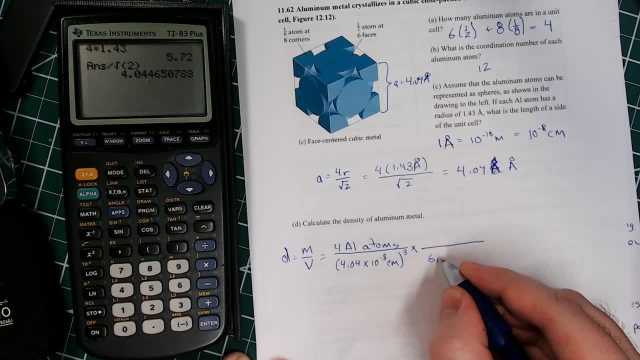 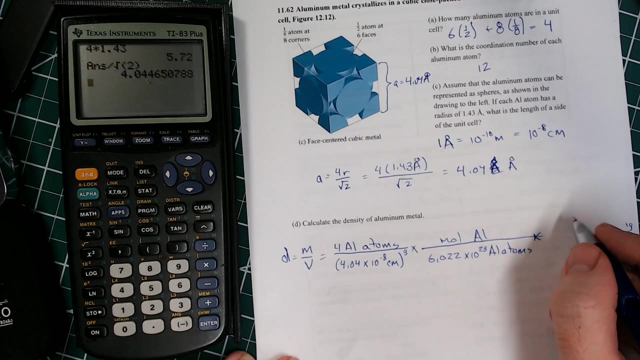 use Avogadro's number. So we'll do 6.022 times 10 to the 23rd aluminum atoms per mole of aluminum, And then finally, we want the molar mass of aluminum. So here I've got my periodic table. 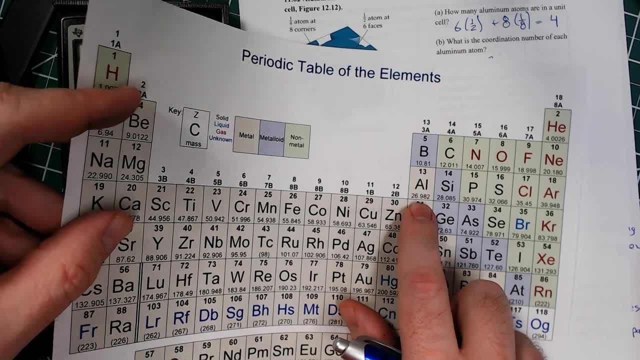 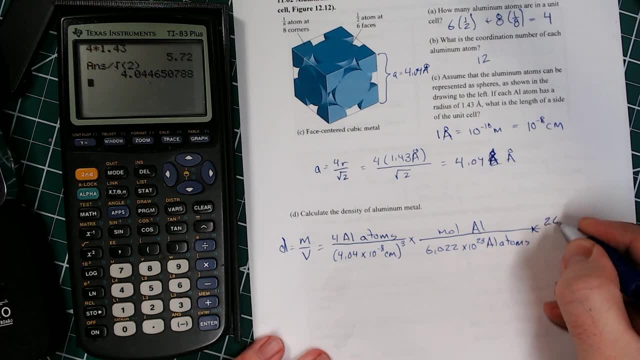 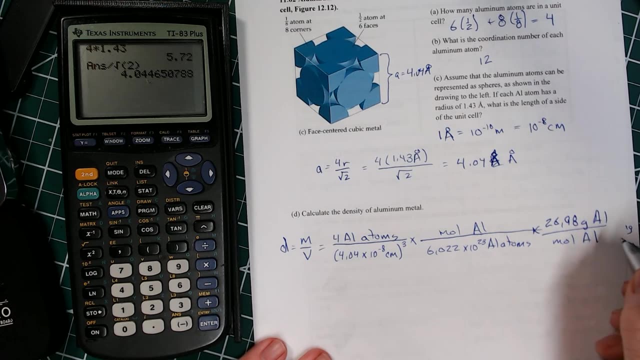 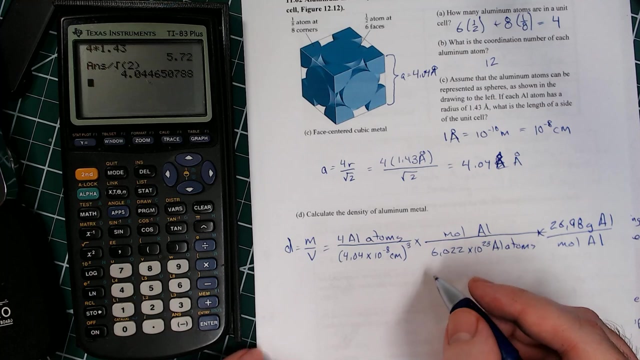 26.98 grams per mole. So we'll put 26.98 there. 26.98 grams of aluminum per mole of aluminum. You'll see the moles of aluminum cancels out, the aluminum atoms cancels out and we're going to get grams per cubic centimeter. 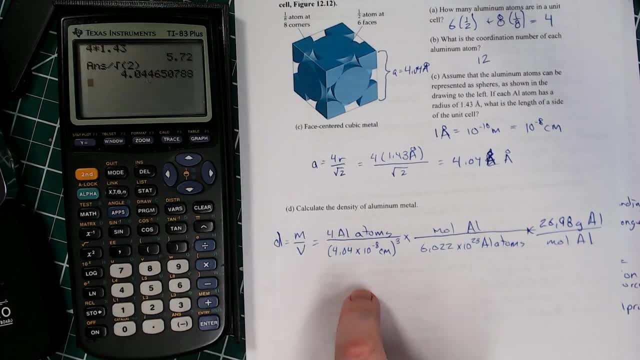 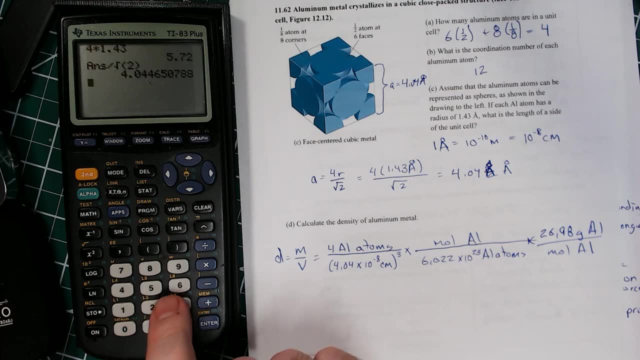 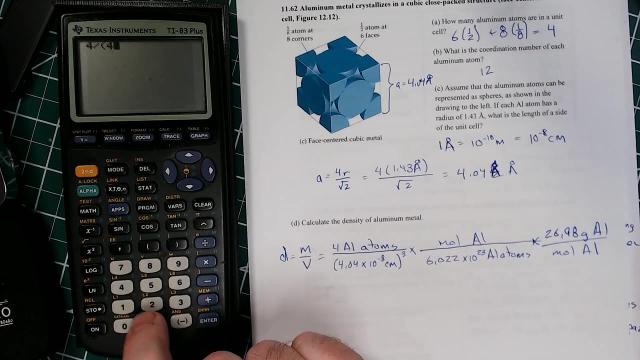 All right now, probably the most important thing to remember is that we're going to get is making sure that you punch all of this into your calculator correctly. So I'm just going to clear that, and we'll put 4 divided by, and then I'll put 4.04. 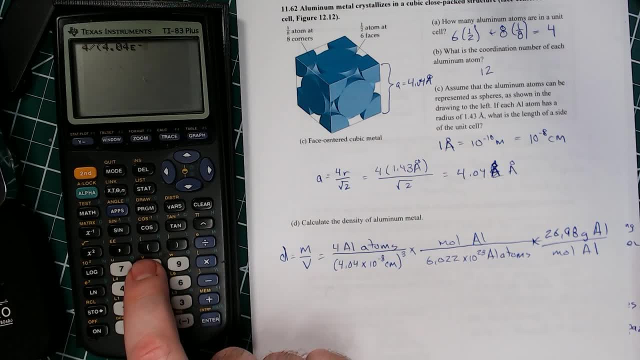 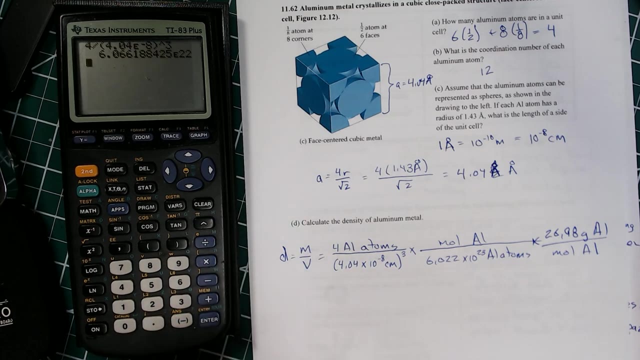 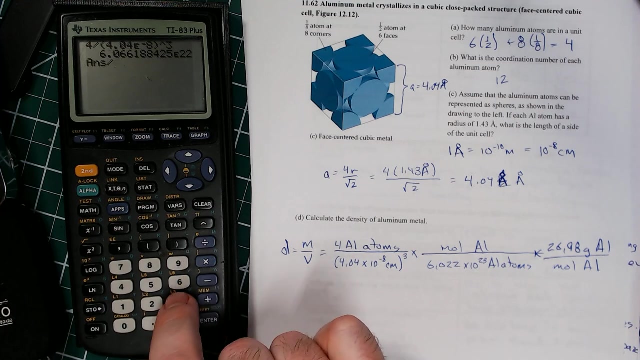 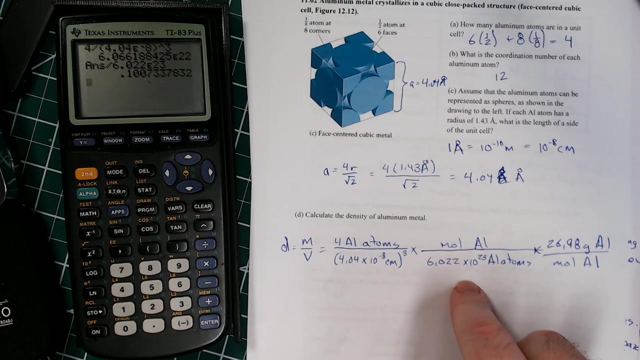 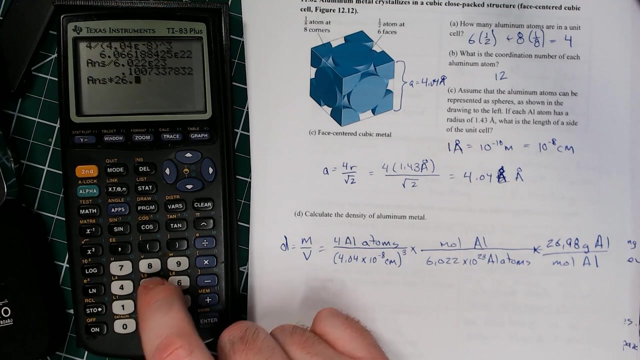 second ee negative 8, close parentheses, and we want that to the third power. All right, so that's this number. Now we want to divide by Avogadro's number. So divide by 6.022. second ee 23.. All right, and now we want to multiply that by 26.98.. So times 26.98. 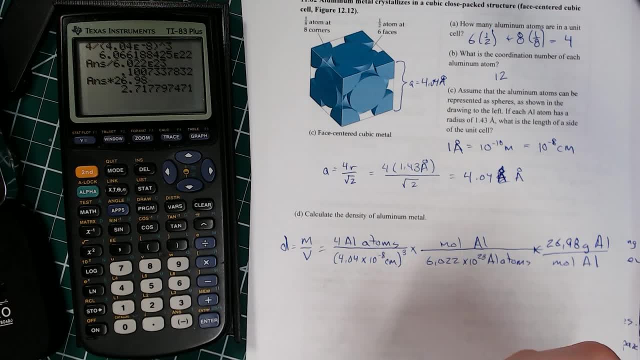 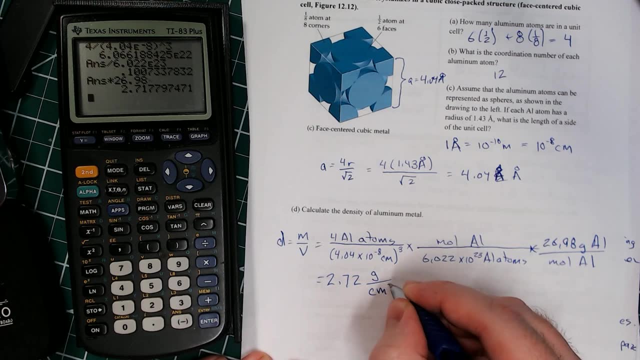 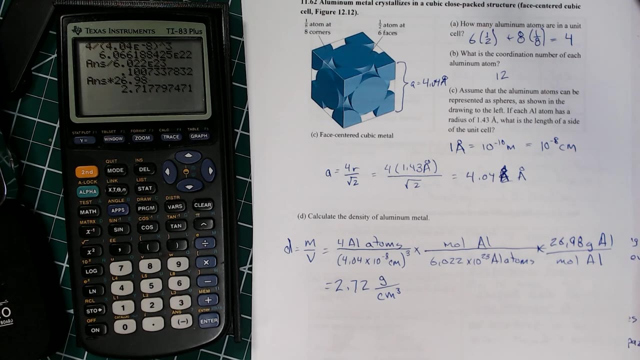 And that gives us 2.72, we will call it So 2.72.. So 2.72 grams per cubic centimeter. All right, So we've got one last or a couple of little details here. not one last thing, a couple. 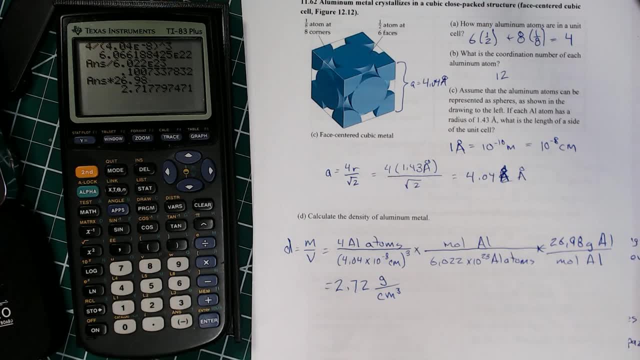 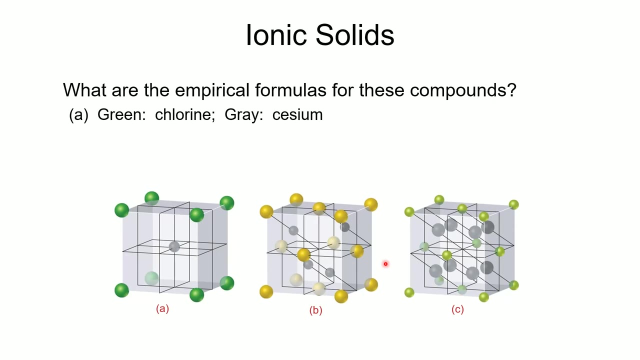 little details. If we've got ionic compounds, it turns out we can determine the empirical formula for an ionic compound by looking at. here we go All right. So we can determine the empirical formula for an ionic compound by looking at a unit cell and determining what, determining what the formula is with 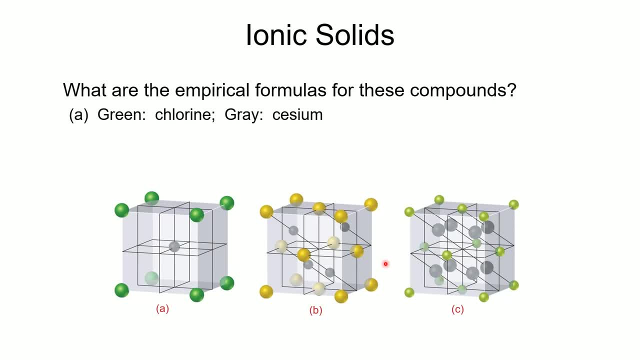 that unit cell. So we're going to start with this green and gray one here on part A. So on A, here we've got green is chlorine. So the arrangement of those green atoms is is gonna be primitive cubic. So each of the green atoms is at the corner. So 1, eighth. 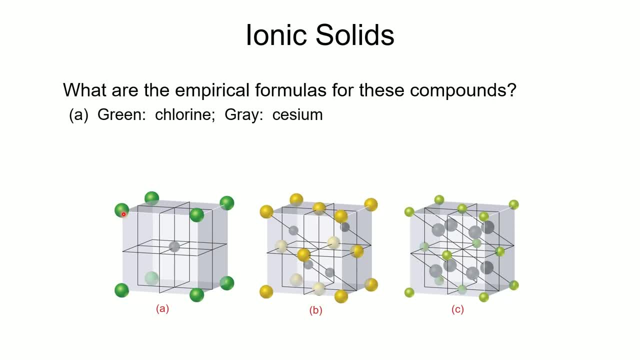 of the atom is within the cell. 1, eighth times eight is equal to one, So there's one green atom, And you'll see here that the cesium atom is right there in the middle, And so it is completely within the cell, And so that means that the ratio of chlorine to cesium 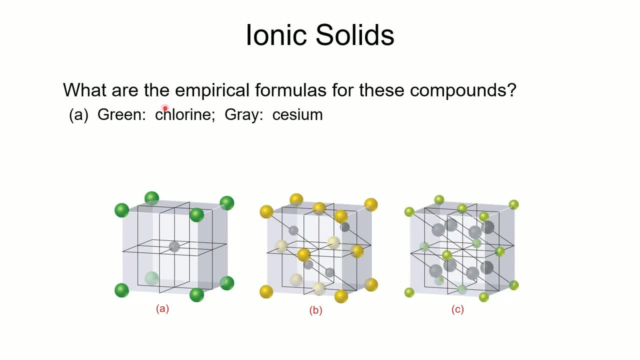 is 1 to 1.. So that means that the formula for caesium and chlorine are 1 to 1.. So we, for cesium chloride, should be CSCL. now, of course, you guys could have figured this out in a different way, because I'm going to come back over here to to this. 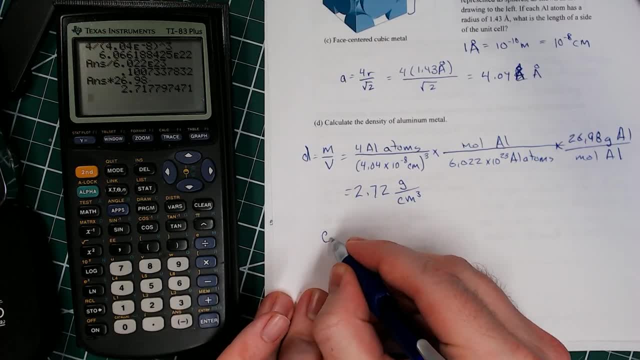 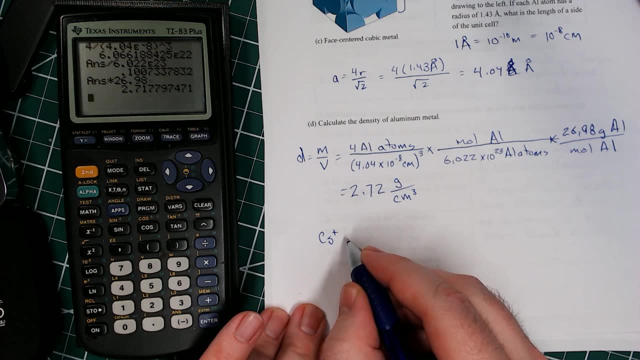 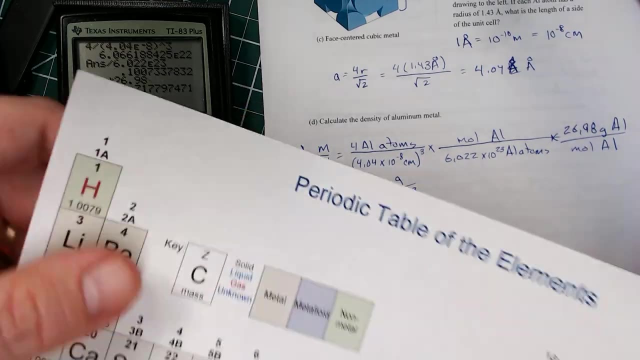 page, because you know that cesium. you know that cesium is in group one, so it has a positive one charge, and chloride is in group seven, so it has a negative one charge. just so everybody's clear. and there's cesium over there in group one. 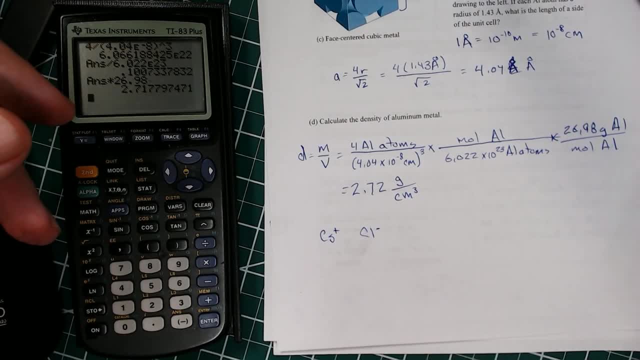 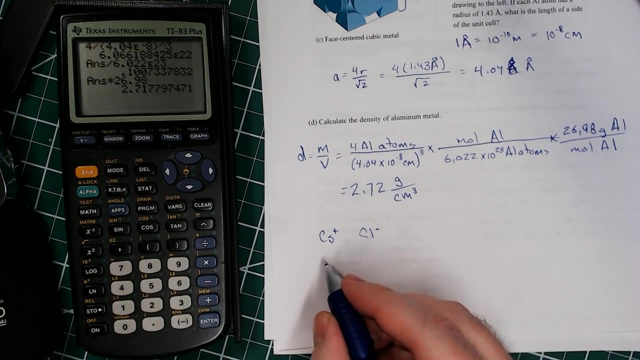 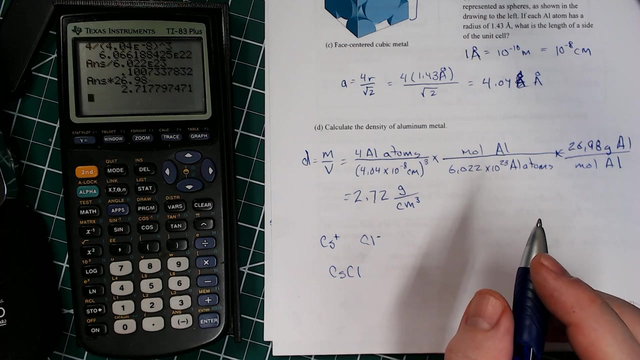 chlorides in group seven, so it has a negative one. so with those, since it's one-to-one, you would have known you would add CSCL. but what this method does is it provides us another way of coming up. you know you're going to have a positive charge and you're going to have a 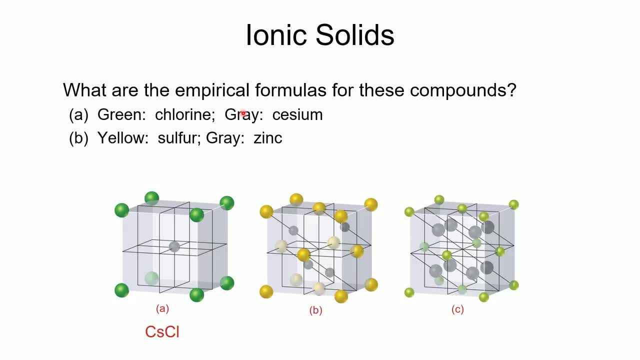 another way of coming up with the empirical formula. all right, so let's look at zinc sulfide. so the yellow atoms are zinc or, I'm sorry, sulfur. so if we count the number of atoms that are sulfur here, we've got 1- 8 at each of the 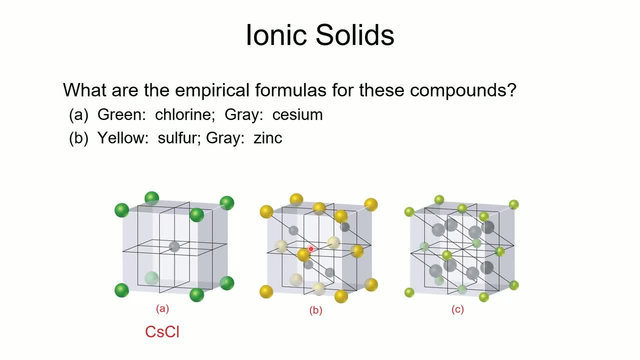 corners. this is a face centered cubic arrangement of the yellow atoms. so one at each corner, 1, 8 at each corner and then half of an atom at each of the six faces. so that means there's four of those yellow atoms that are within each cell. so 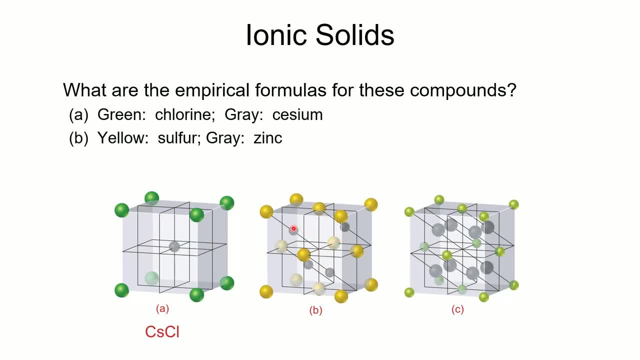 the net number is four for the gray atoms. it's a little bit difficult to see here, but this gray atom is in between this corner and the middle of that unit cell. this one is in between this face and the, the edge there, and so we will find that that that all four of the zinc atoms are within the cell. so that means 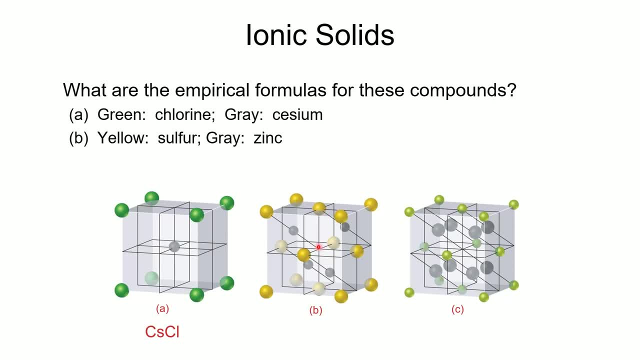 there's a four to four ratio. so the formula is: it's not going to be ZN4S4, it's going to be just ZNS, the lowest whole number ratio. so ZNS, all right. and then finally, here, the green ones are calcium. so you'll see, that's face centered. with face centered, that's four atoms. the gray: 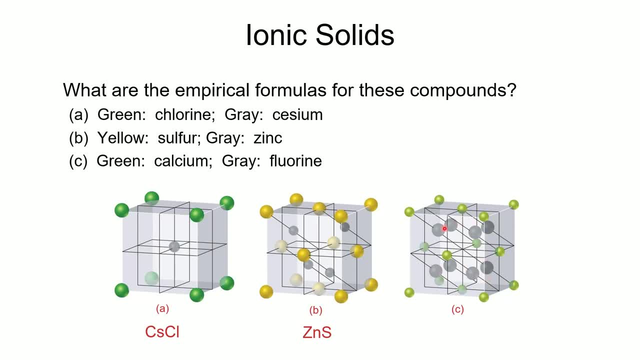 ones are fluorine or fluoride ions, and you'll see that all eight of those are within the cell. so it's a four to eight ratio. four to eight is one to two, so it may take two to three. uh, so one calcium for every two fluorines. it'll be ca f2. 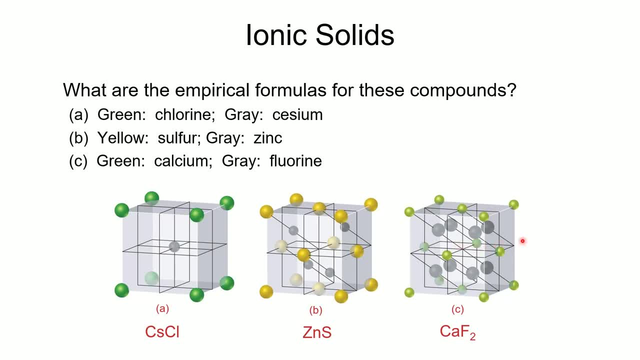 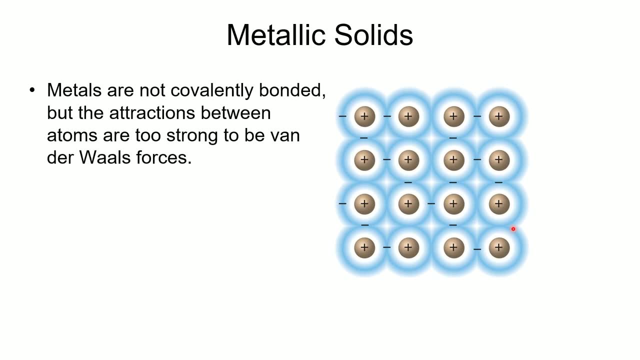 it'll be ca f2, so that's something that I want you to be able to do, all right. one last little topic here is talking about metallic solids. metallic solids are different, then. they're different than covalent bonds, they're different than ionic bonds, so the electrons aren't transferred and it's not like the. 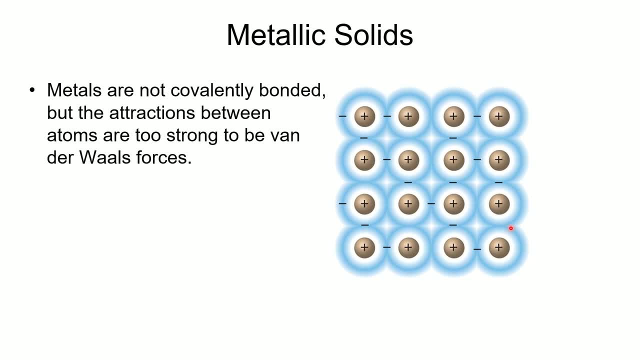 and atoms. the electrons are shared among all of the atoms, And so your valence electrons can move freely from one atom to another. As a consequence, that means that metals are really good conductors of heat and electricity because those electrons can move so freely. All right, So they are.